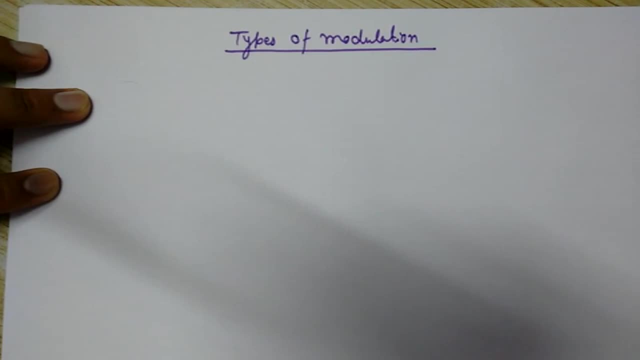 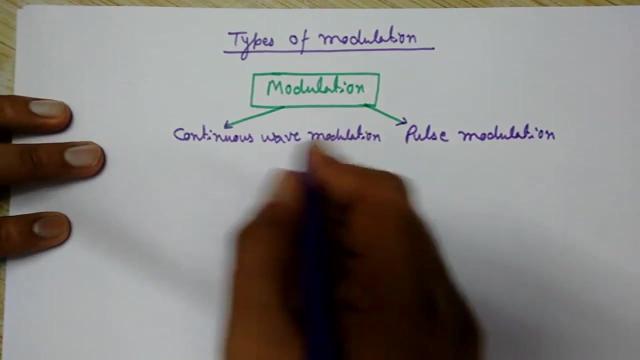 see different types of modulation one by one. So this modulation can be broadly classified into two categories: The continuous wave modulation and pulse modulation. What is the continuous wave modulation? In continuous wave modulation, the carrier wave is continuous. In this, the carrier wave is continuous, While in case of pulse modulation. 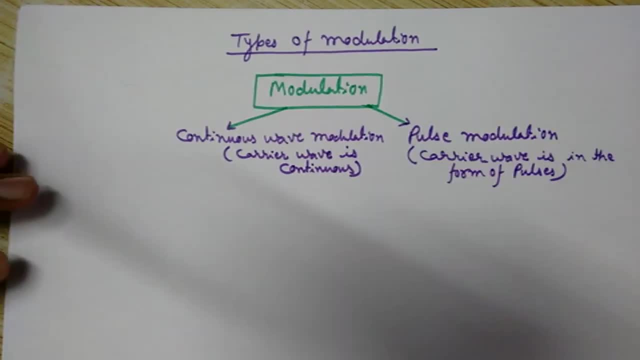 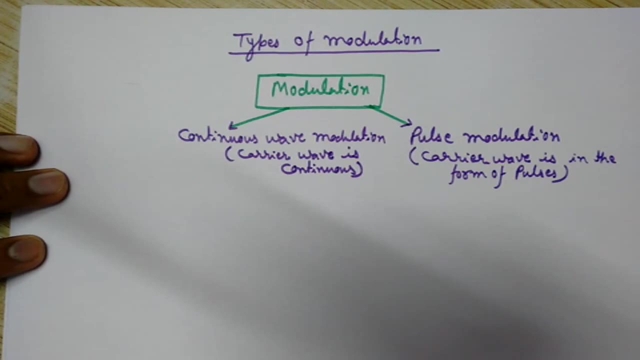 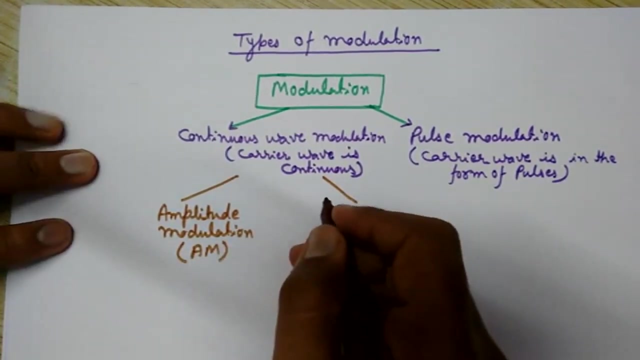 the carrier wave is in the form of pulses. This continuous wave modulation again can be classified into amplitude modulation and angle modulation. There are again two types. We can write it as aM and another is angle modulation. We can again classify this angle. 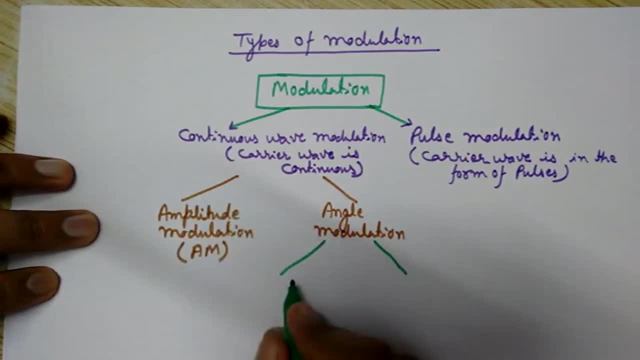 modulation into two types. These are the frequency modulation and phase modulation- Phase modulation denoted as fM. Then this is pM, the phase modulation. So these are two typesALK OUT���. könnten wir小�itations stellen? 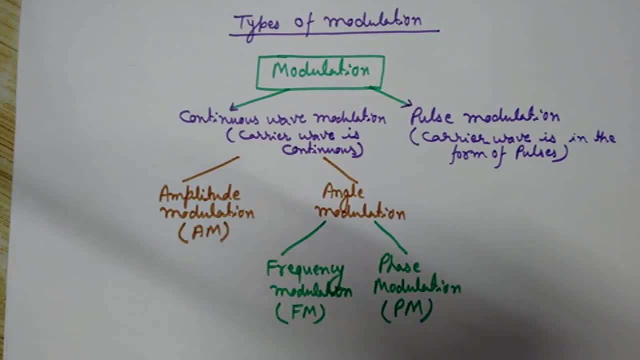 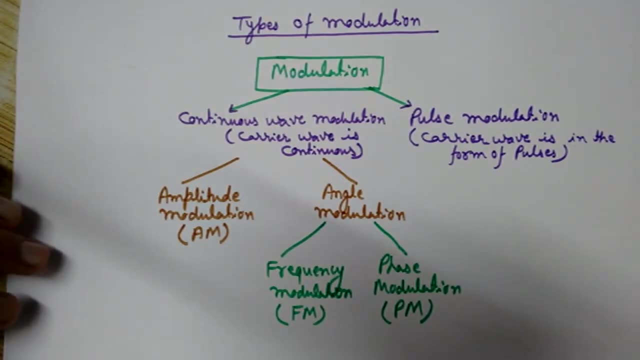 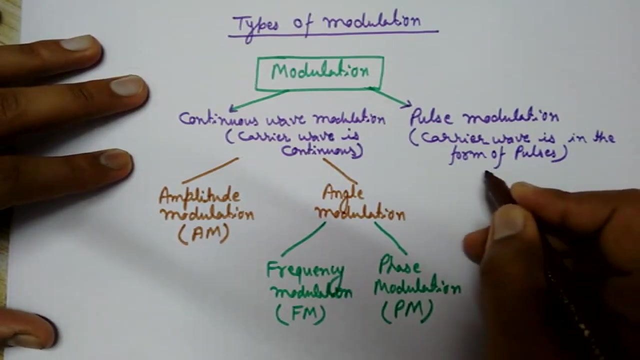 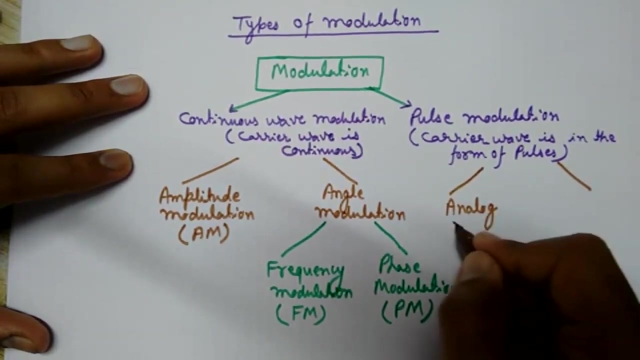 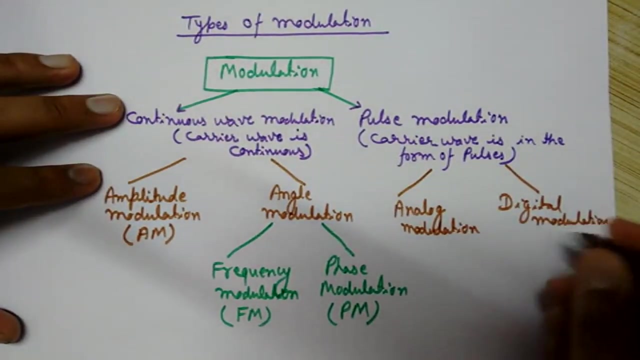 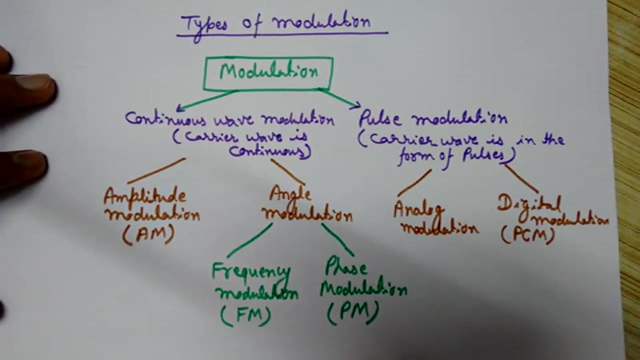 are the two types, okay, of angle modulation. now we will see types of pulse modulation. the pulse modulation can be classified again into two forms. this one, the analog and digital. two forms are analog modulation, analog and digital modulation. these are the two forms. an example of digital modulation is pulse code modulation, PCM. we will discuss it later and the types of analog. 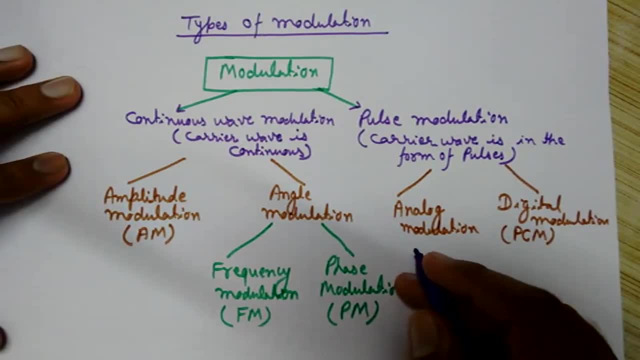 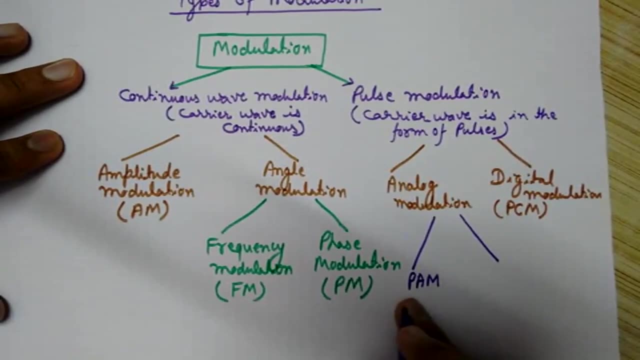 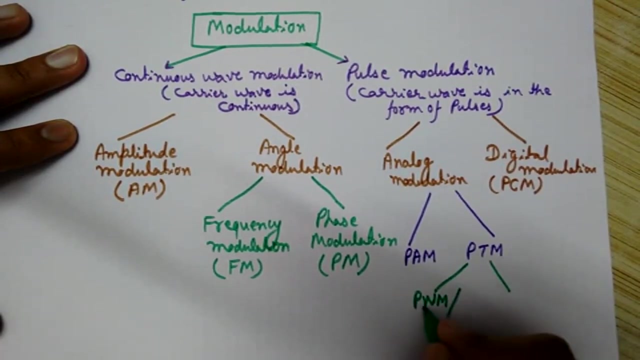 modulation are. we can broadly classify them into two types. P a m stands for. it stands for pulse amplitude modulation, and the second one is PTM means pulse time modulation. this pulse time modulation can again be offered two types. the P W M means pulse width modulation, or also called as pulse duration modulation. 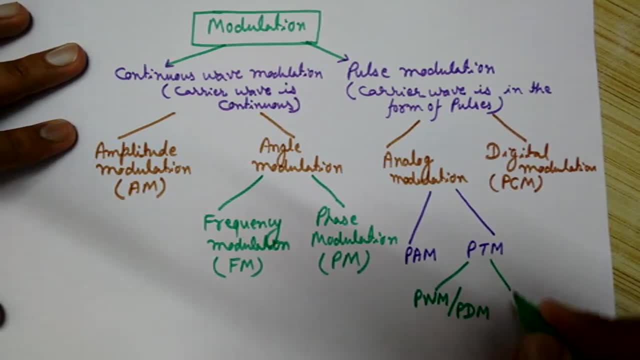 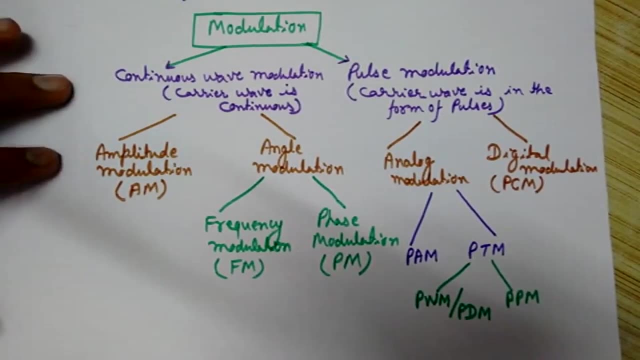 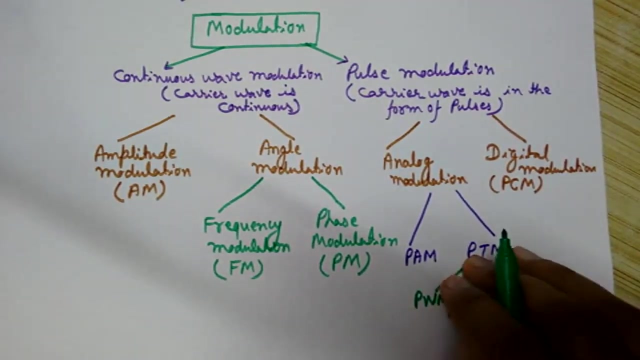 okay, and the second one is PPM: pulse position modulation. so these are the two types of this: pulse time modulation, pulse width or pulse duration modulation. this is the same thing and the pulse position modulation. so this is very important classification. you should keep this in mind always. we will discuss these. we will discuss these in the next class. we will discuss. 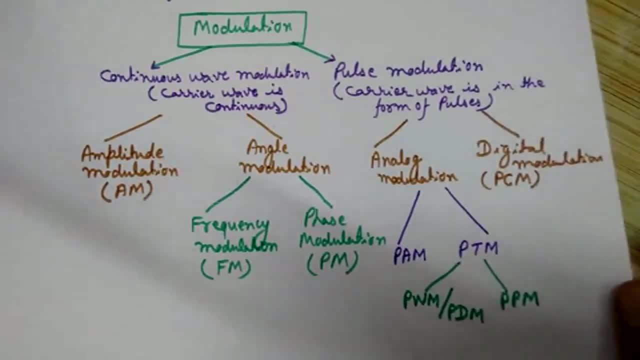 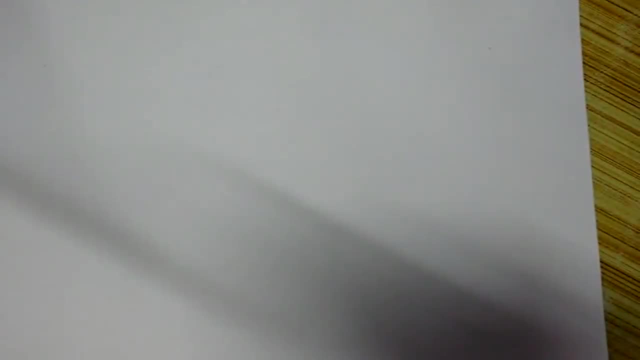 each one of these modulation types in some detail, not in very depth, but we will introduce each one of these. so let's start with the amplitude modulation. the first one is the amplitude modulation. amplitude modulation called as am. so the amplitude of a signal means the value that is. 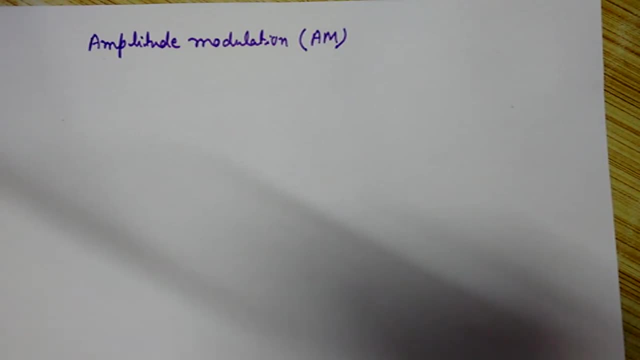 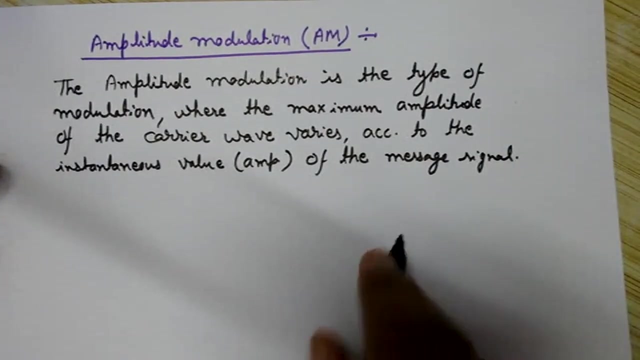 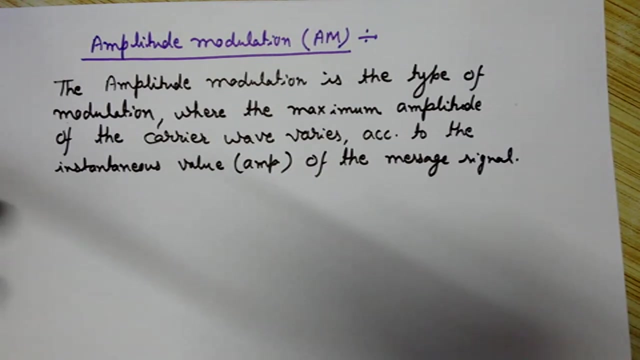 That is the magnitude of the signal. This is the amplitude. So let's define what is amplitude modulation. The amplitude modulation is the type of modulation where the maximum amplitude of the carrier wave varies according to the instantaneous amplitude of the message signal. Got it? I have already told you that message signal is also known as the modulating signal or the base band signal too. So now I will draw a diagram that will help you in getting the point in a more clear way. 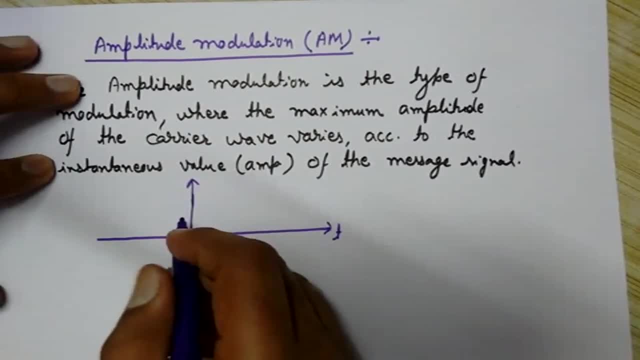 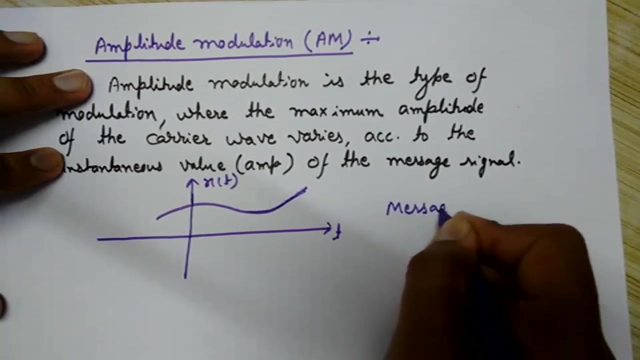 This is the time axis and I am drawing here the signal that I want to transmit. This is the message signal. actually, This is the waveform of the message signal. Let's denote it by xt. and this is the time axis. This is the message signal. 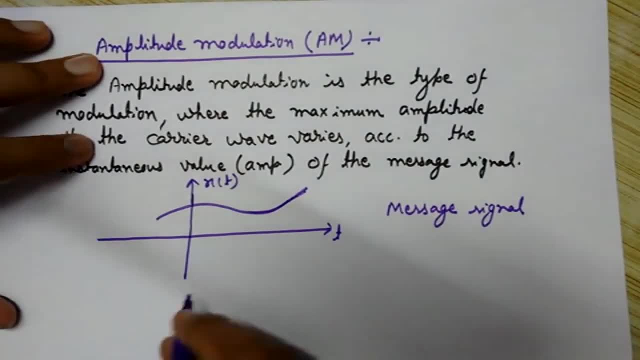 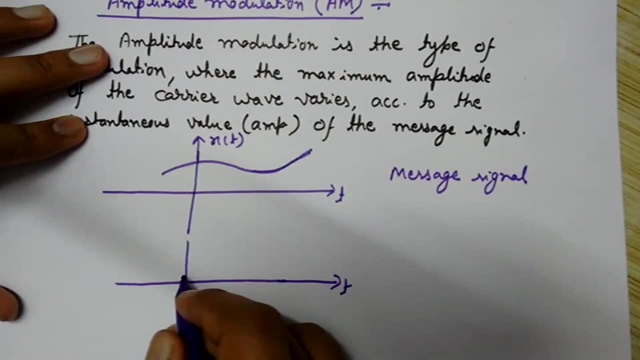 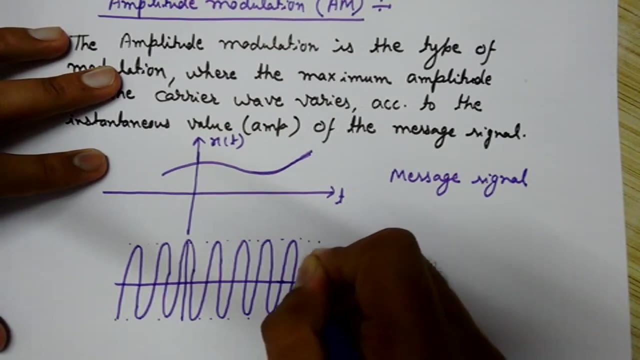 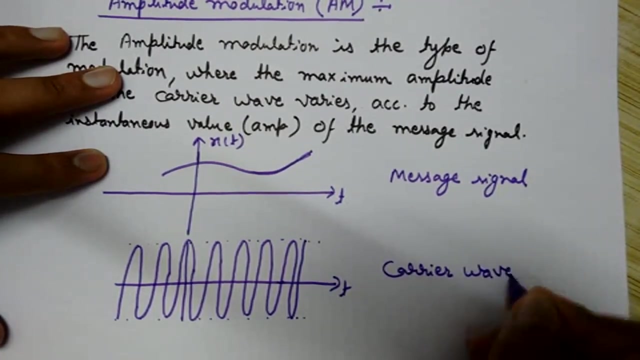 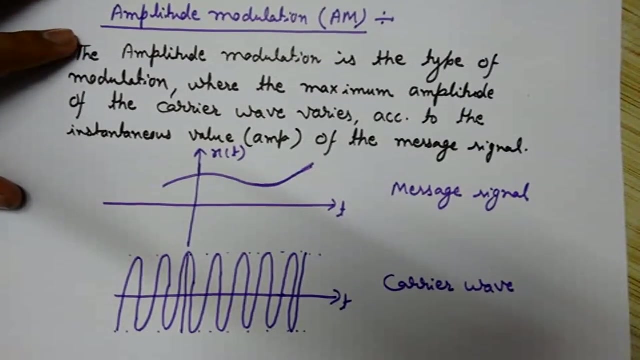 And this one is the carrier wave. Now I am drawing the carrier wave here, This carrier wave, very high frequency. okay, this is the carrier wave. this is a high frequency wave. now, as per the definition that you have seen of an amplitude modulation, you know that the amplitude modulation is the type of modulation we are, the 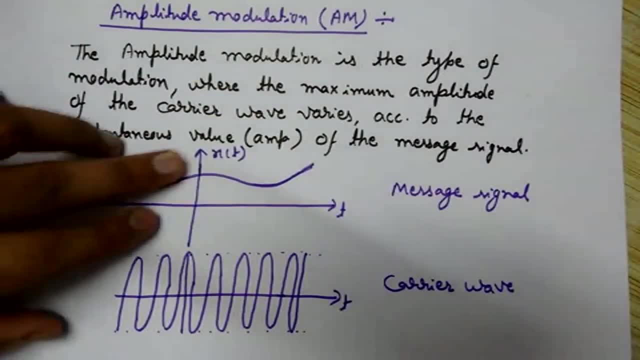 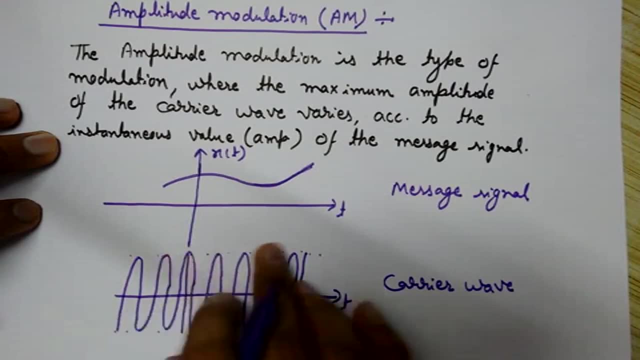 maximum amplitude of the carrier wave varies according to the instantaneous value of the message signal. so we will vary the amplitude of these. the maximum amplitudes of this carrier wave will vary according to the shape of this message signal. so let's see how does this happen. I will draw the modulated. 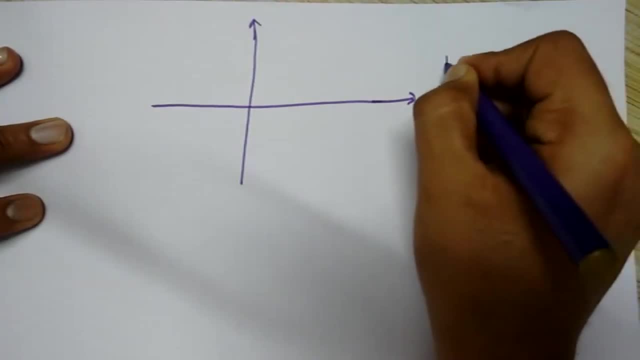 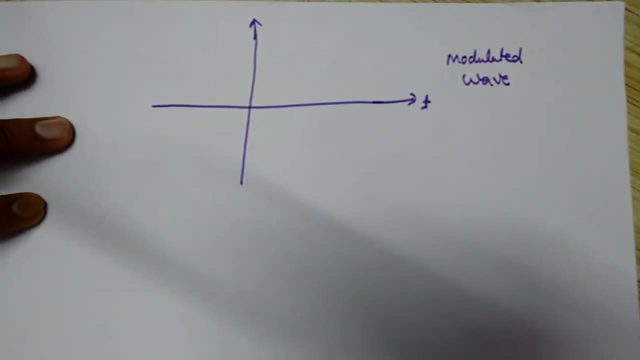 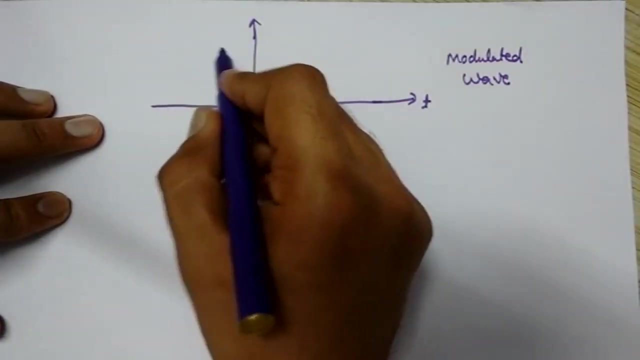 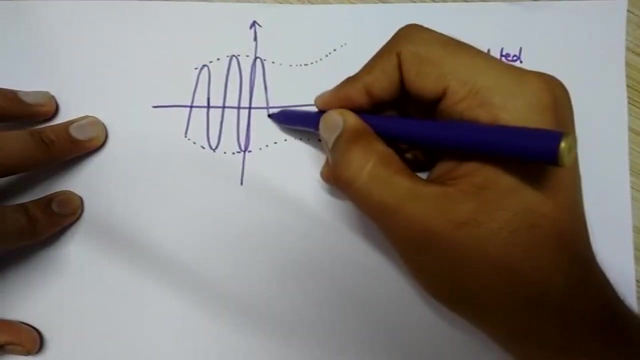 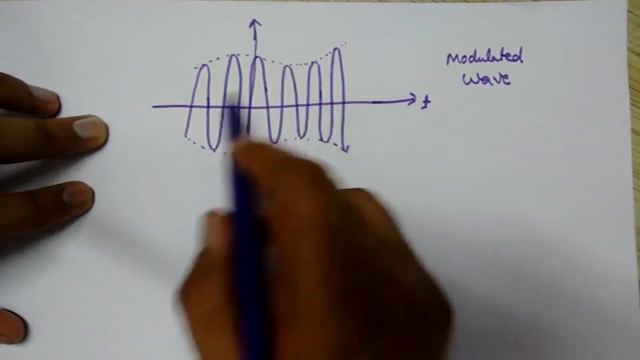 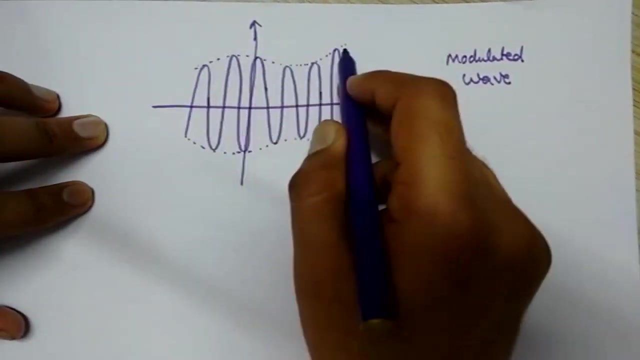 waveform, and I'm here drawing the modulated waveform. modulated wave or the modulated signal we obtain after modulation. so this is something like: okay, this is the waveform. as you can see, this is the carrier wave. okay, this is the carrier wave, as initially it was having the constant amplitude, as you. 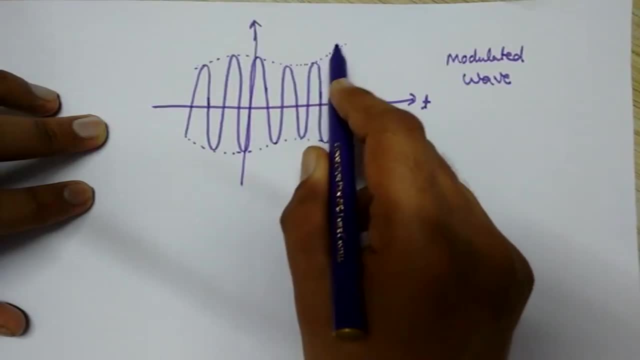 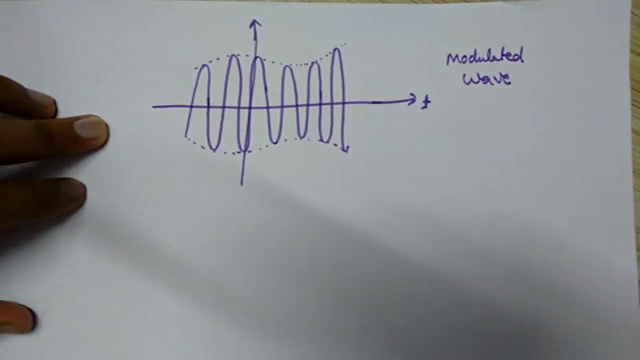 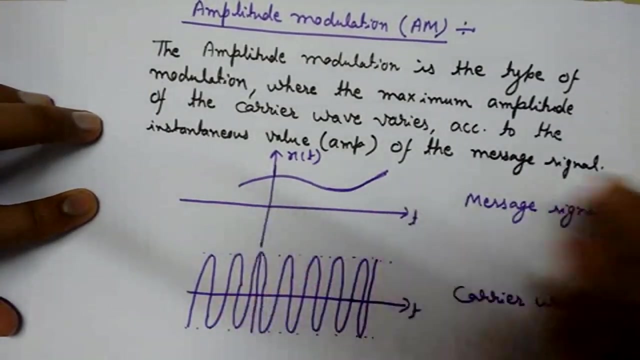 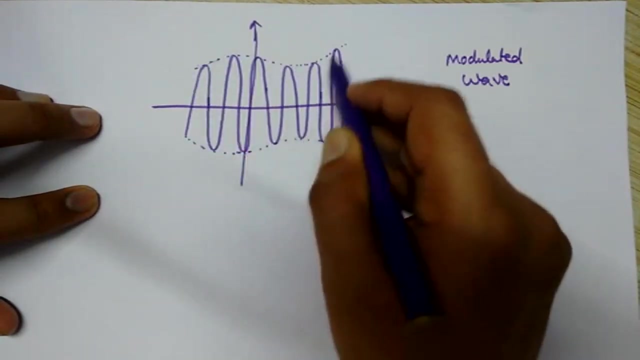 have seen earlier. but now I have varied this. the maximum peaks have varied as per the shape of the our original message signal. as you can see here, this was the message signal. the shape of this variation in the maximum amplitude of the carrier wave is as per the shape of the message signal, so we call this these. 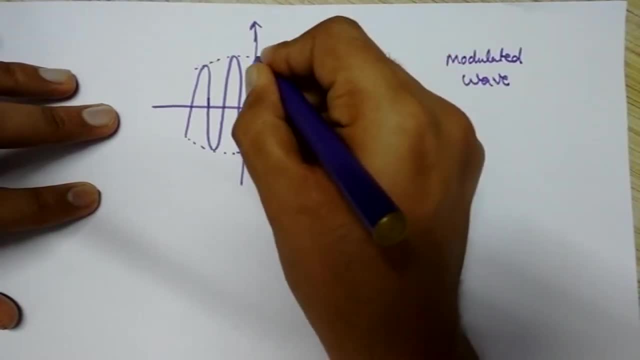 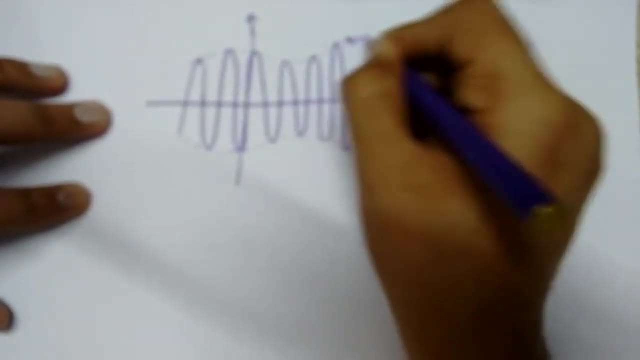 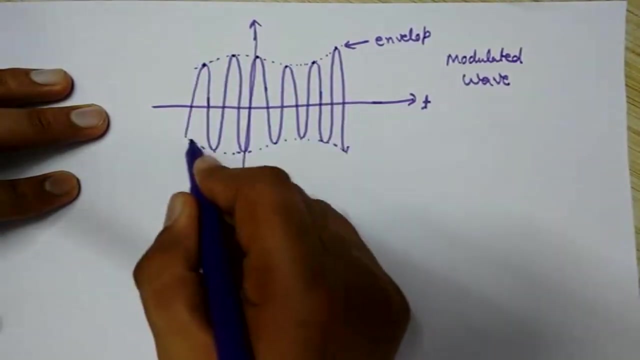 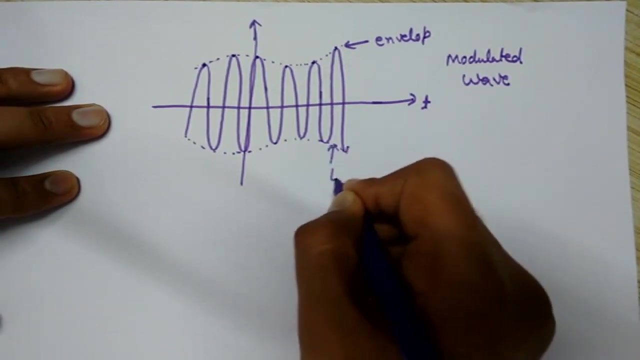 two- this is shape- is obtained by touching the peak peaks of this signal, so this is called the envelope, envelope of the signal. and, as you can see, these are two identical sidebands. we call this band as the lower sideband and this one as the upper sideband and the 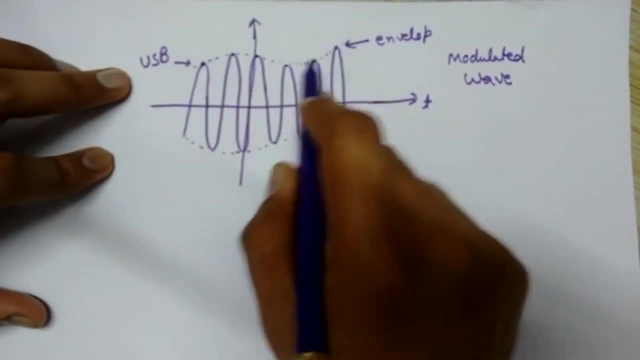 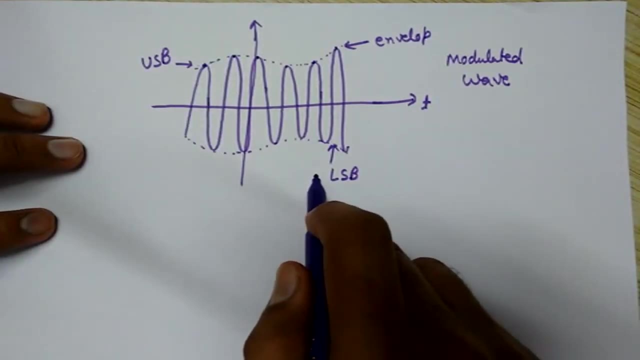 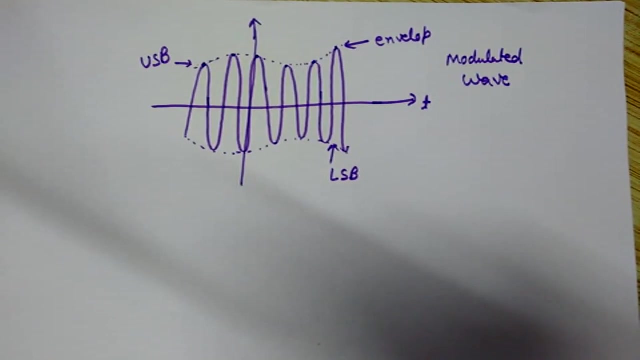 information is contained completely. we have the full information in this band and also in this lower sideband. we can get information from any of these two envelopes, either upper sideband or lower sideband. so these sidebands have the message signal in it in the form of amplitude variation. 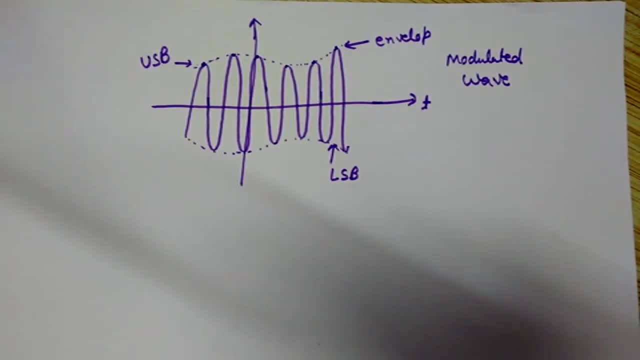 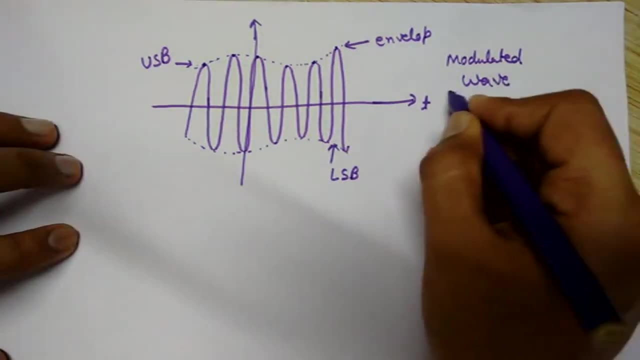 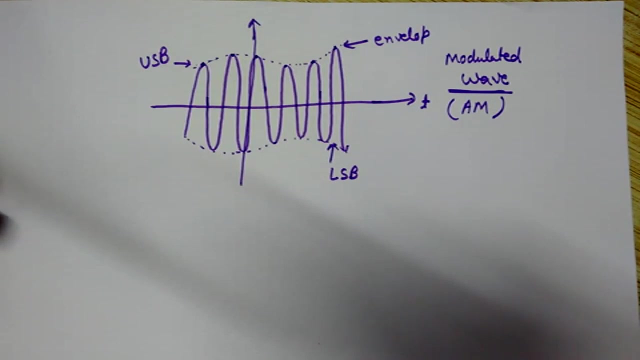 of the carrier wave. I hope you got the concept of amplitude modulation. this is the modulated wave, actually the amplitude modulated wave. now we will discuss the another type, frequency modulation. what is frequency modulation? it is denoted by FM before seeing the frequency modulation, and we will 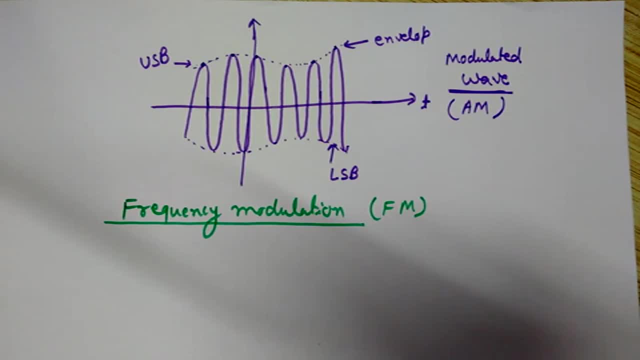 see what is frequency. so the frequency of a wave means the number of complete wave cycles passing per second. it is also denoted by 1, by T. if this is a simple waveform, then this is the time period up from here to here. this is the time period of the complete cycle of this wave. 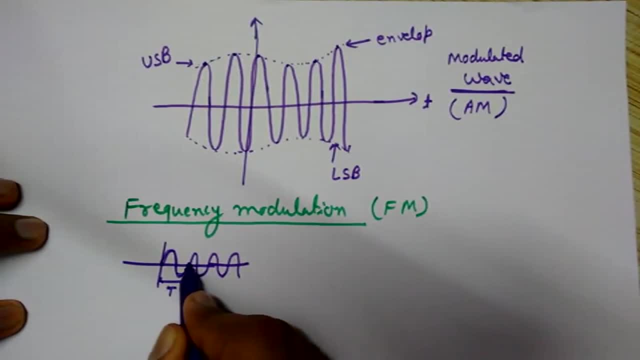 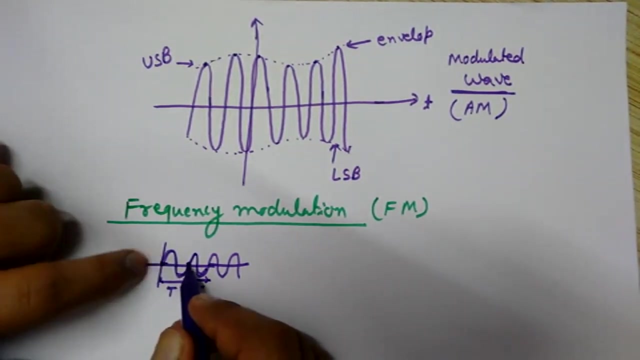 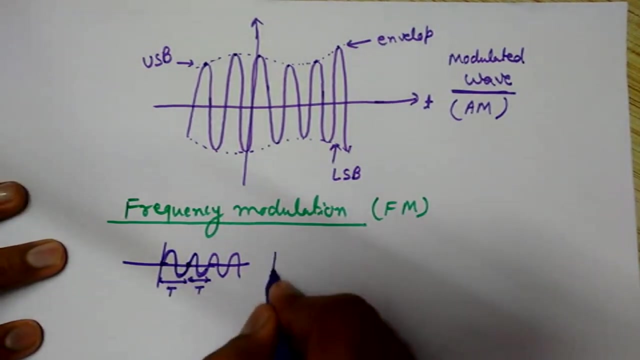 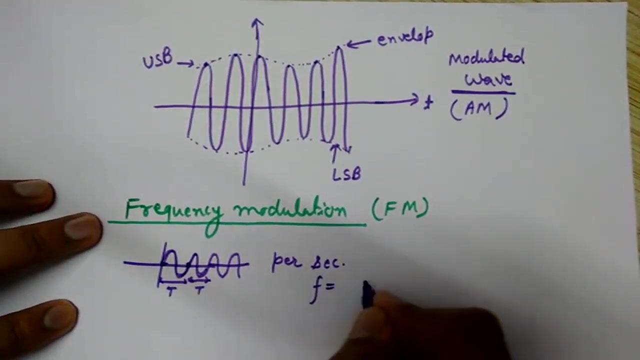 because after this time period this wave repeats it. so this is the another. from here to here is another time period, so this from here to here is the one cycle of this waveform. so the frequency means how many such cycles are passed per second. per second. okay, so this frequency is also denoted as 1 by time. it's inversely proportional, or it is equal to 1 by T of 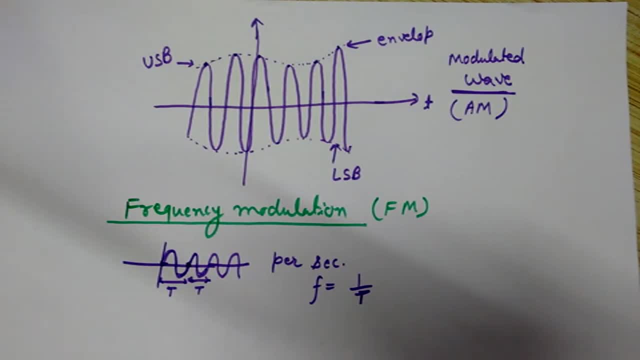 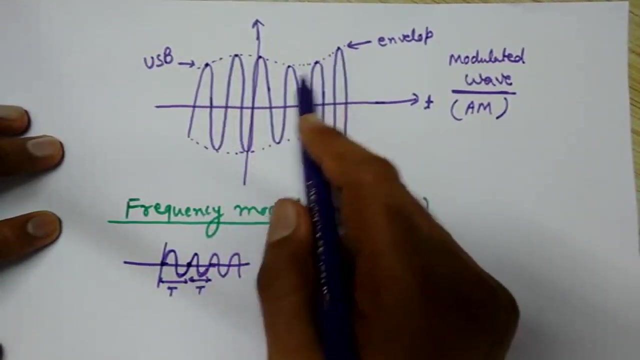 the frequency. so now let's come to the definition of frequency modulation. in frequency modulation the frequency of the carrier wave is varied according to the amplitude of the message signal, here the. in this example we have seen in amplitude modulation that this variation of carrier wave was in the form of amplitude of it we varied. 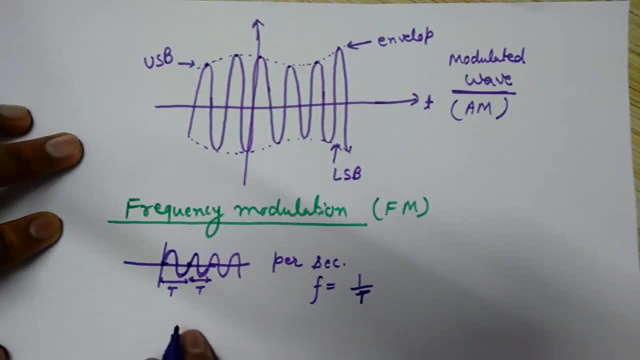 the amplitude of the carrier. but in this case, in this frequency modulation, we will not change the amplitude of the carrier wave, but we will just vary the frequency. so the information will be contained in the variations of the frequency of the carrier waves. I think I'm clear. so let's write the definition. 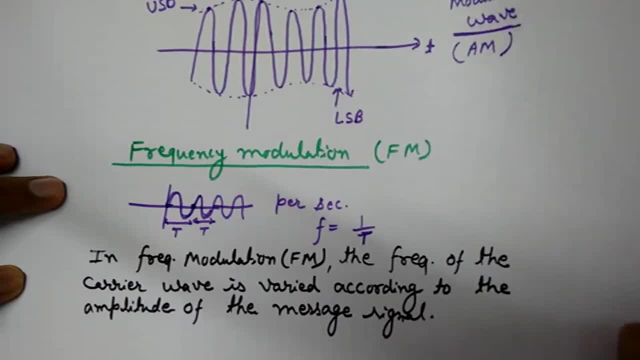 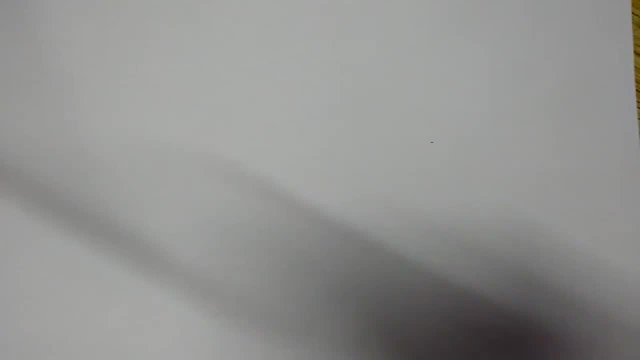 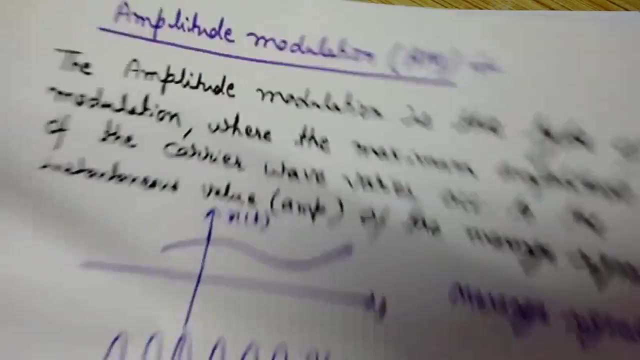 here. I have explained it to you already now. we will see it with the help of a beautiful diagram. how does this happen? I will draw the same diagram. I don't want to draw it again. so we are taking this modulating signal again. this is the message signal. 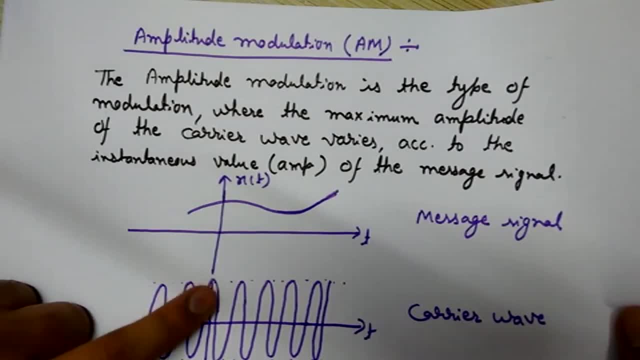 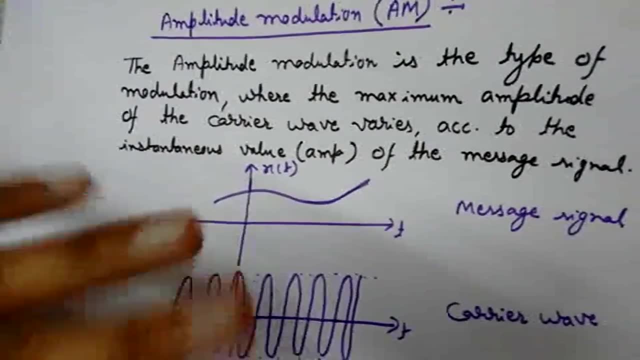 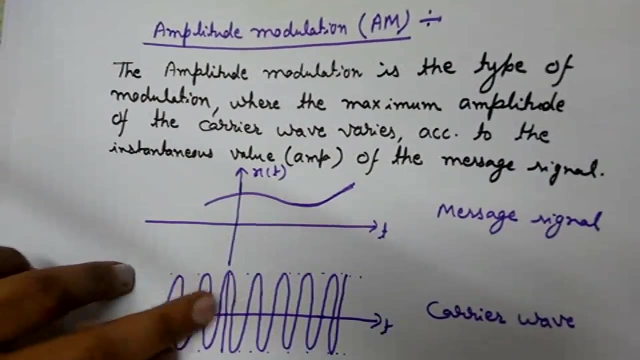 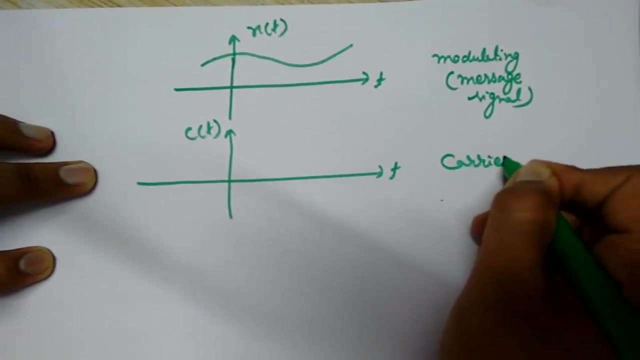 signal that you want to transmit, and this one is a carrier wave. this was the example of AM, but our we are considering these two waves. so in this modulation, in FM, in frequency modulation, we are going to vary the frequencies denoted by XT, we can denote it by CT, the carrier wave. this is the carrier wave having a high 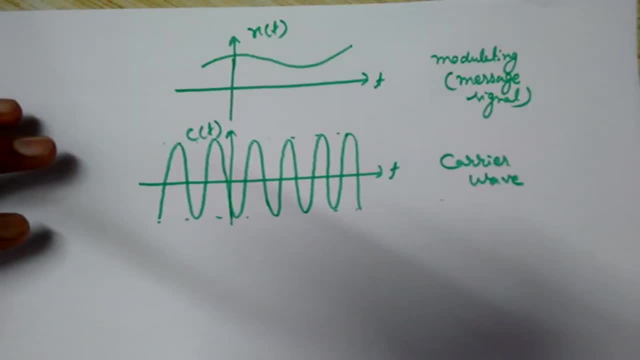 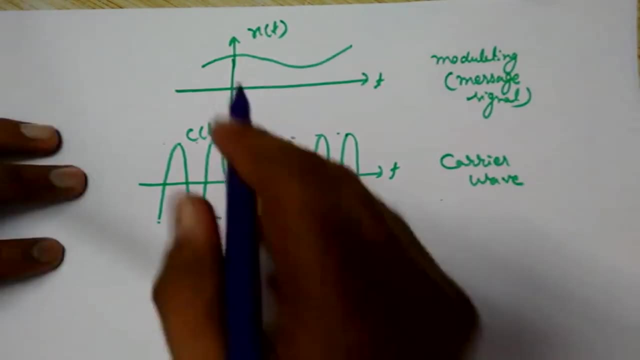 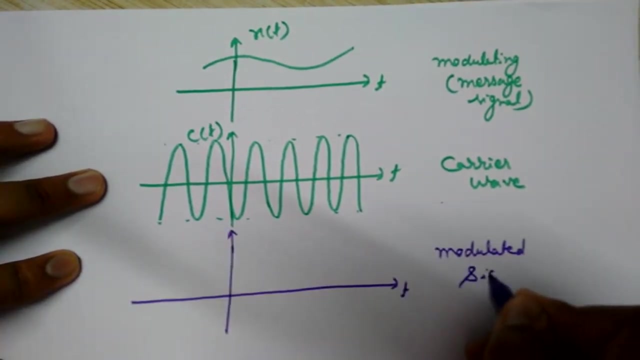 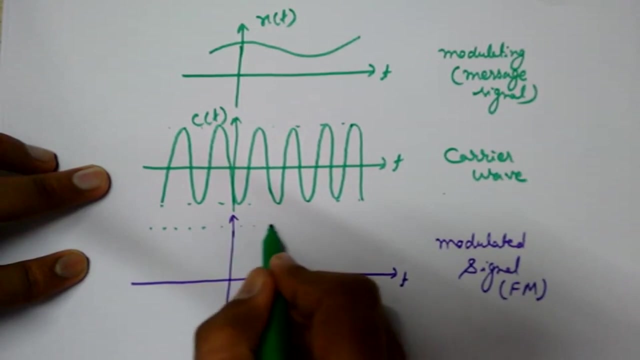 frequency, and constant high frequency and it's very the frequency of the superior babe, as per the variations in the amplitude of this message. signal, as see it, modulated, see now, that is FM, the frequency modulator. signal, as I told you, that the amplitude will not change, only the frequency and the frequency of the. 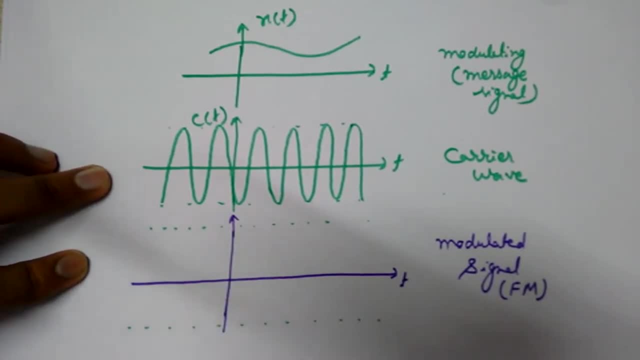 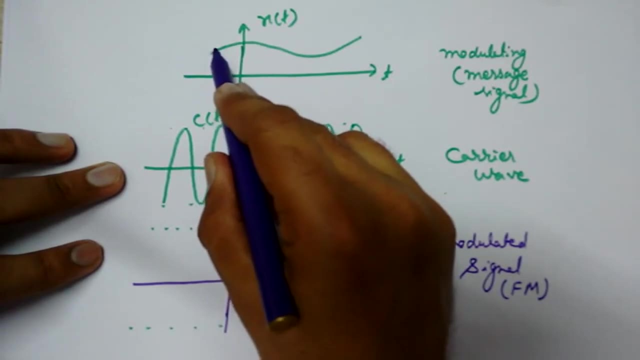 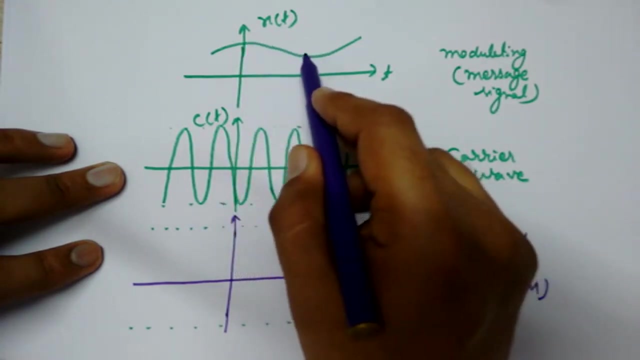 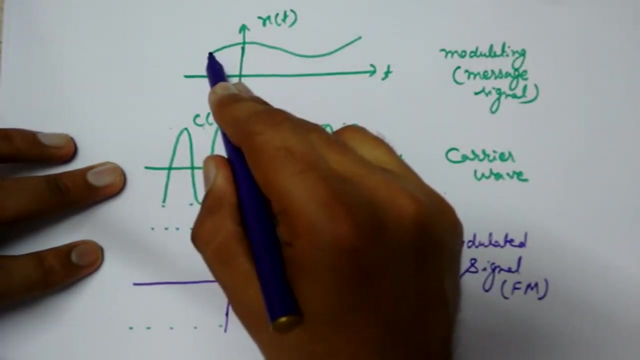 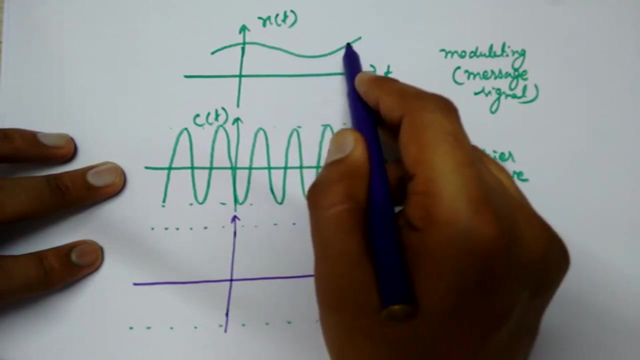 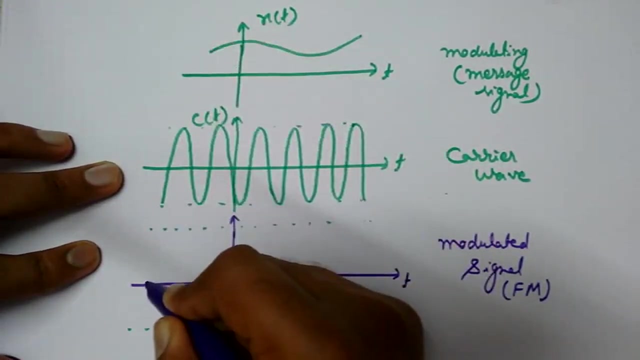 Now the carrier wave will be changed, So I'm keeping it constant. Now let's see here, Here we can see here that the amplitude is increasing maximum. at this point It is decreasing and then again it is increasing. So our frequency of this wave will start from certain frequency, Then it will increase, Then the frequency will decrease, Go to minimum and then it will again start to increase. So here it is, at some frequency. 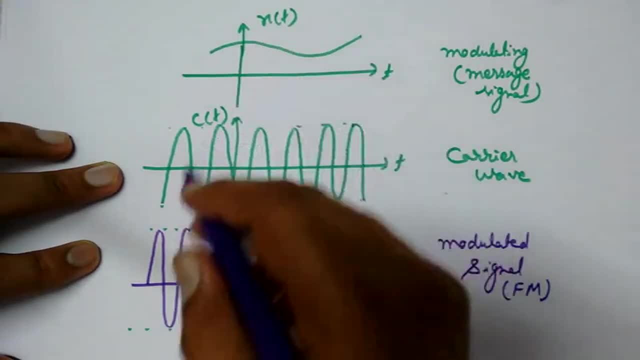 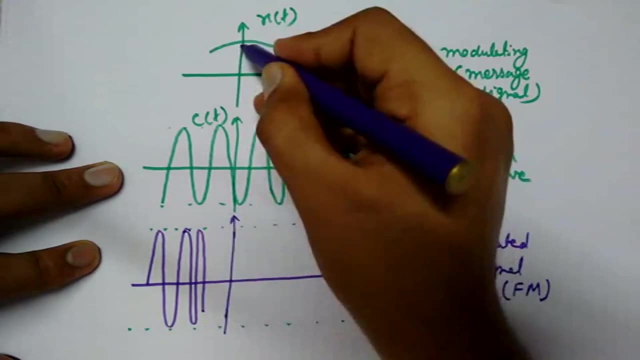 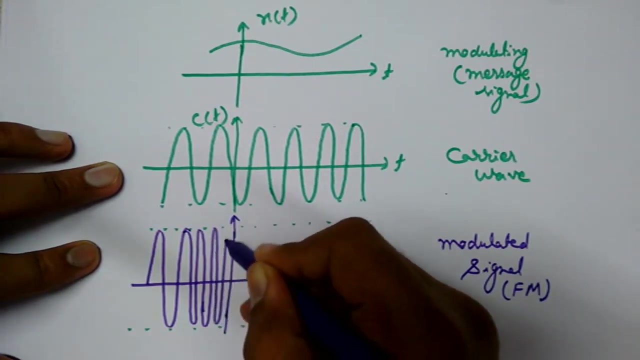 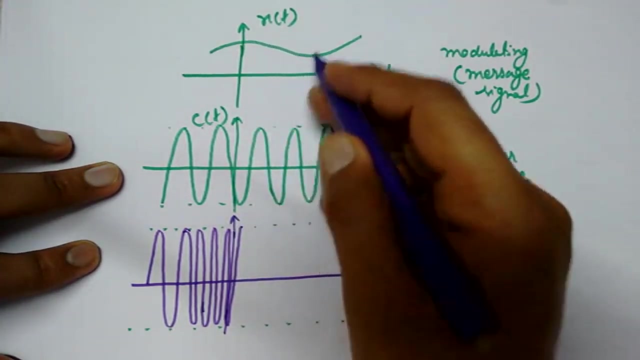 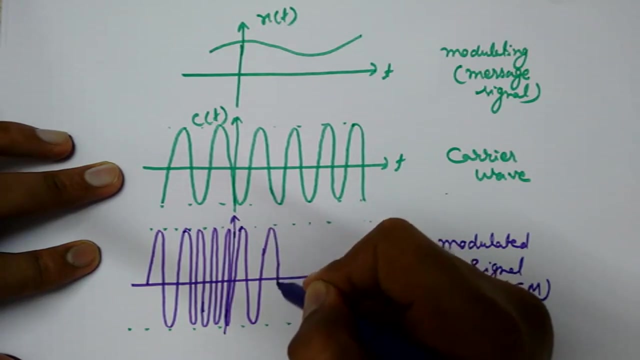 Okay, It starts to increase. So at this point it is maximum. I'm just drawing the rough diagram, so don't mind it. And it is again. it again starts to decrease. It means the spacing between the waves will increase as the frequency is decreasing. 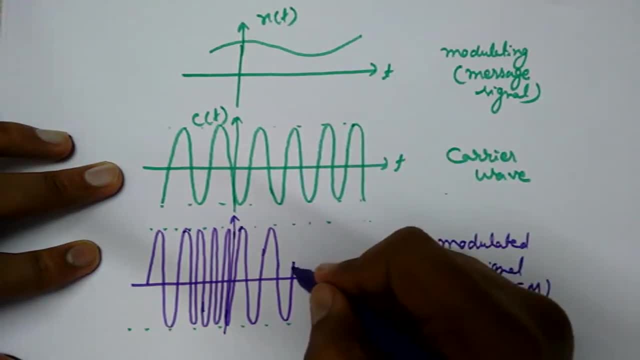 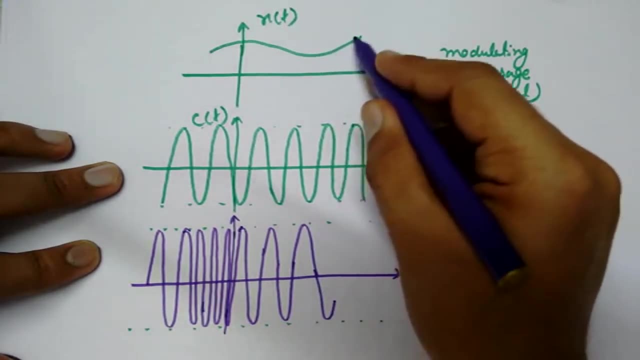 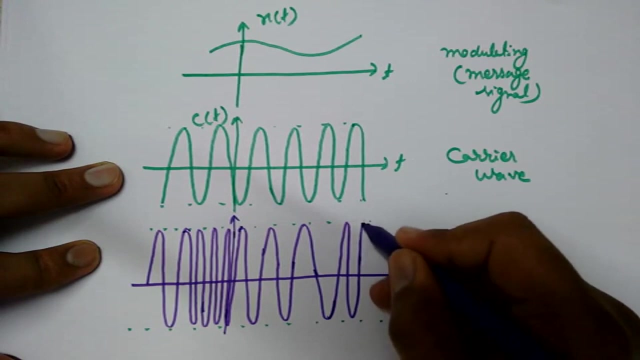 At this point it will be minimum. The frequency will be minimum means the spacing between the waves will increase and again it starts to increase At this point. so the spacing will reduce again. Continuously it will reduce. It is going to reach to the peak. 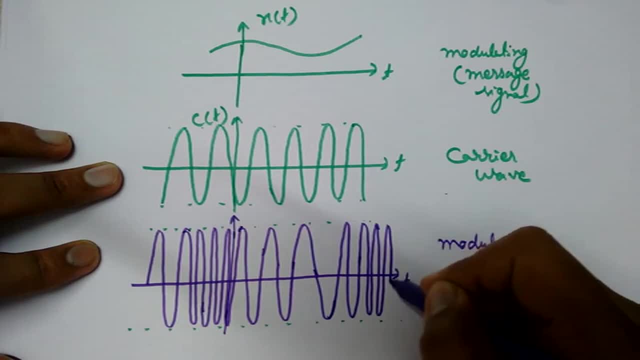 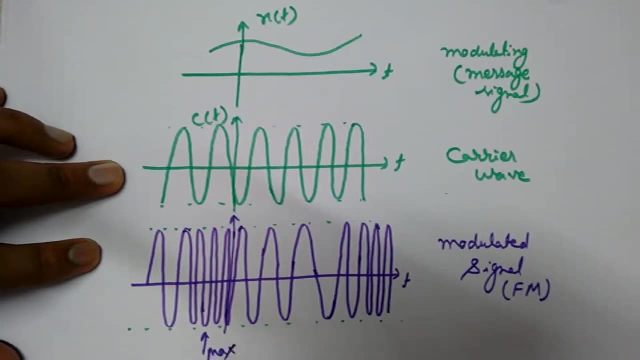 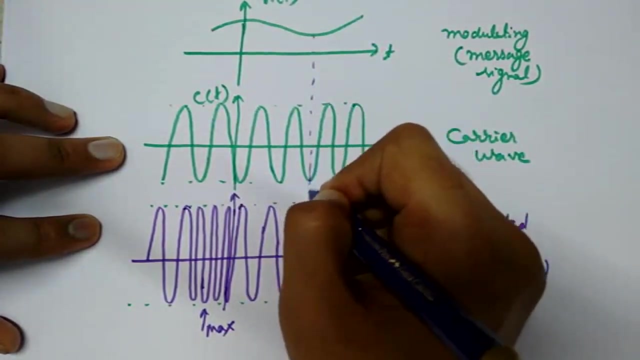 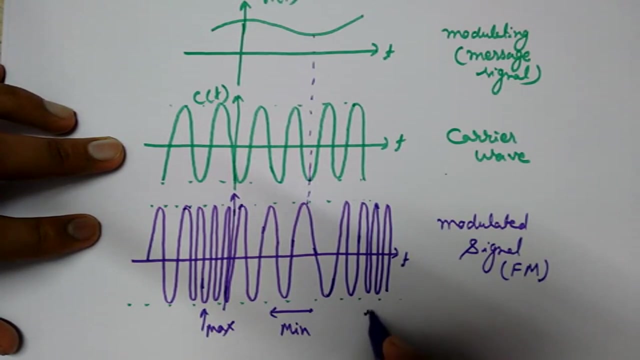 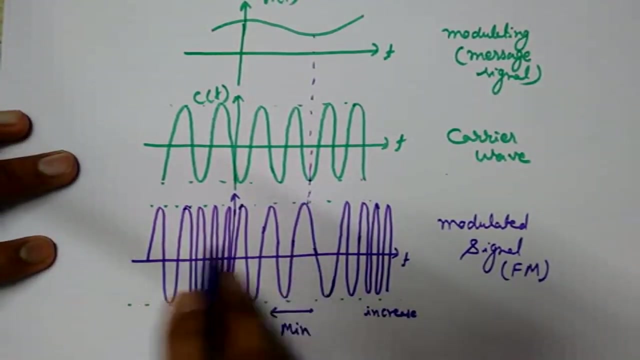 So it will decrease the spacing. So frequency is maximum at this point And you can see that here frequency is at minimum. Okay Again, here it again increases. So I think it is clear. The information is in the form of frequency. as per this, 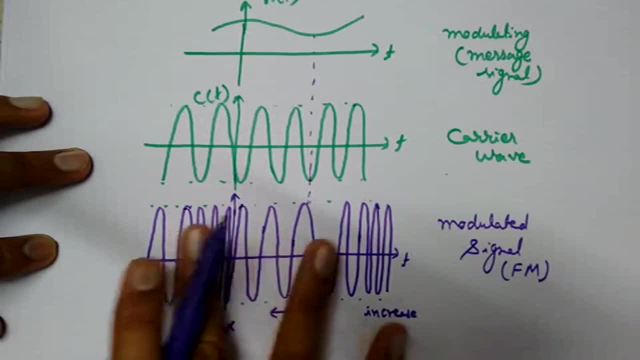 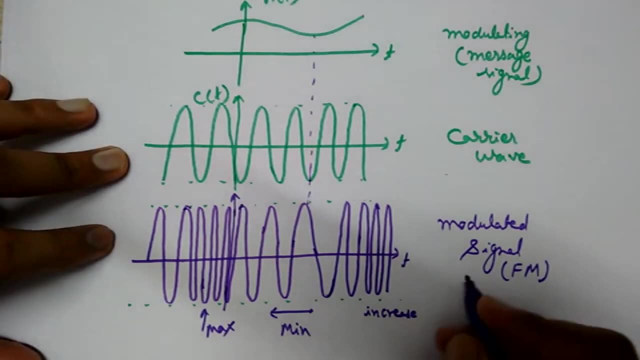 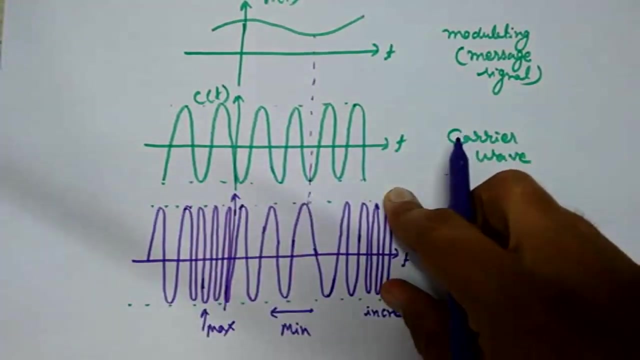 Millions masses. It is varying the frequency, The space hearing between this carrier… This is varying. So here you can also notice here that the amplitude is not varying. here Information is not in the form of amplitude, as was the case in case of amplitude modulation. 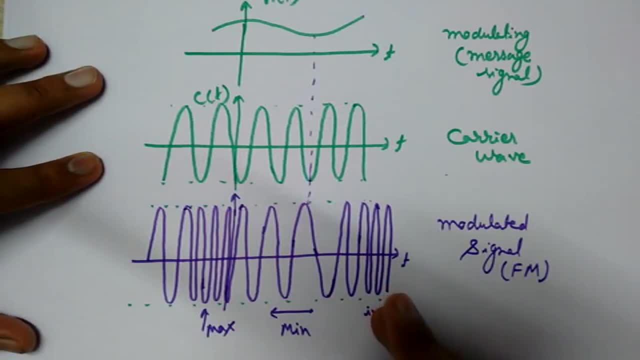 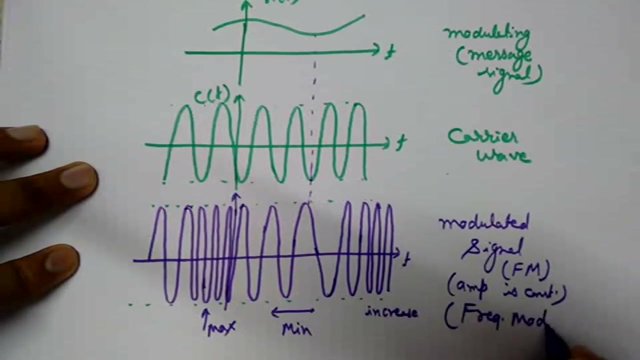 Just the information is contained in the variations of the frequency of the carrier wave. So here the amplitude is variable, is constant. Now the phase modulation. Next comes the phase modulation. I will discuss the phase modulation. This is the frequency modulated waveform First. 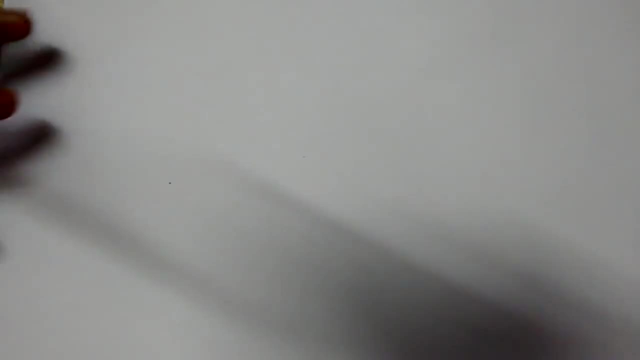 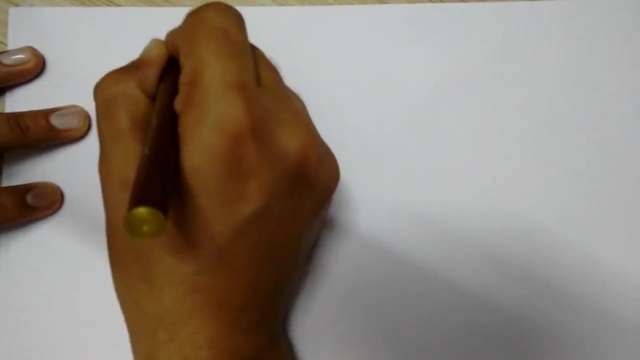 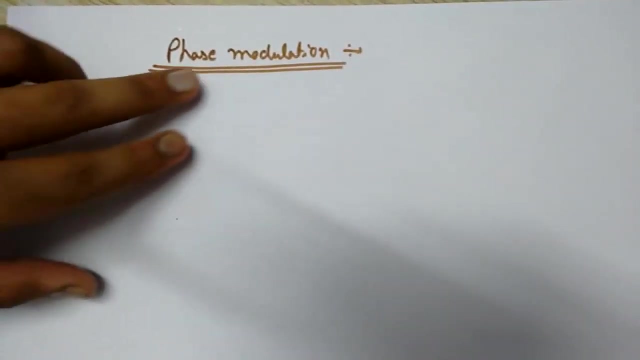 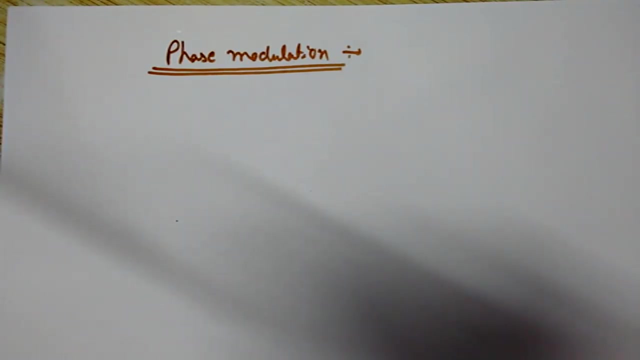 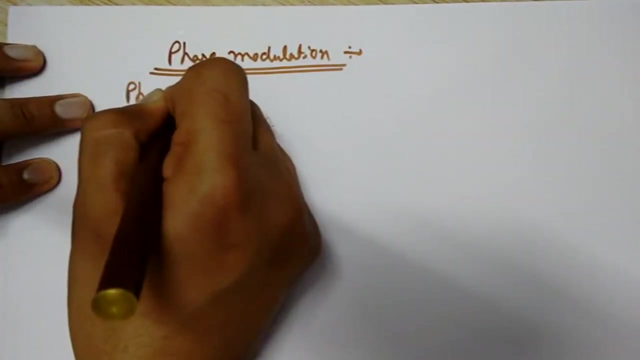 before describing the phase modulation, it is important to understand the concept of phase. What is phase? Let's understand it. What is phase before this? What is phase? Phase is the position of a point at some time instant. What is phase? Phase is the position of a point at 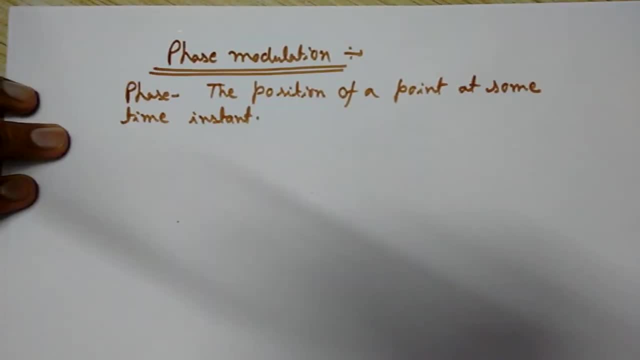 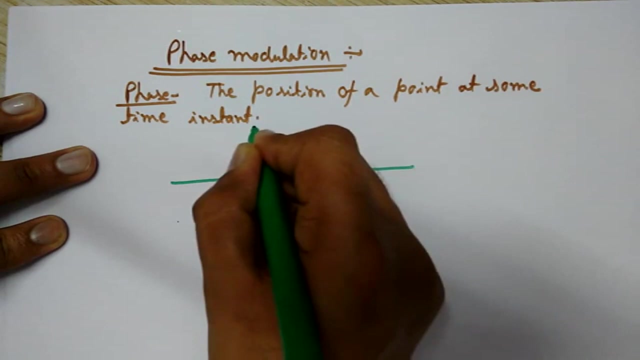 some time instant. some time instant. Let's understand the phase difference. What is phase difference, then? The phase difference is created when a wave moves horizontally on the time axis, When some waveform. let's understand it again with the help of a diagram sketch Here I will. 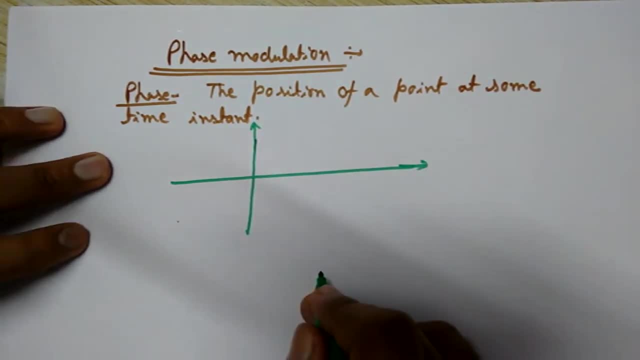 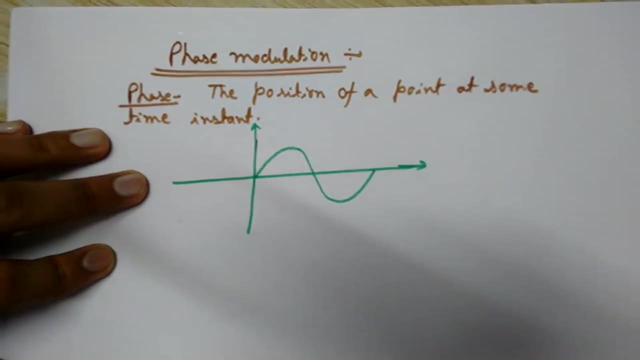 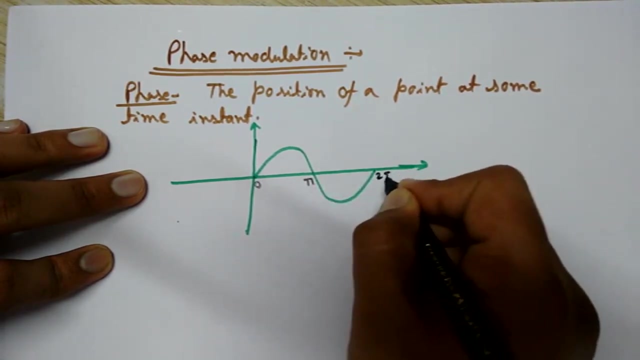 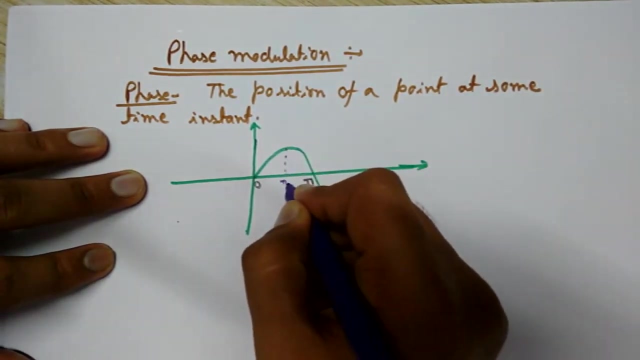 draw two waveforms, two sinusoidal waveforms having some phase difference. You know this point: this is zero, this is a sinusoidal wave. this is zero. pi 2, pi radians: This one is a first wave and this is the pi by 2.. 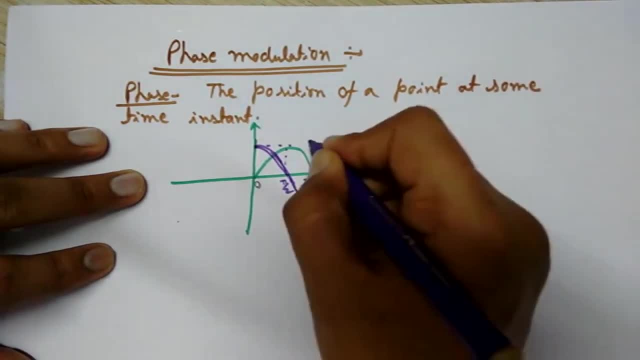 This is a second wave and this is the pi by 2.. This is a first wave and this is the pi by 2.. Another sinusoidal wave. this is the first wave. let's call it first. this one is the. 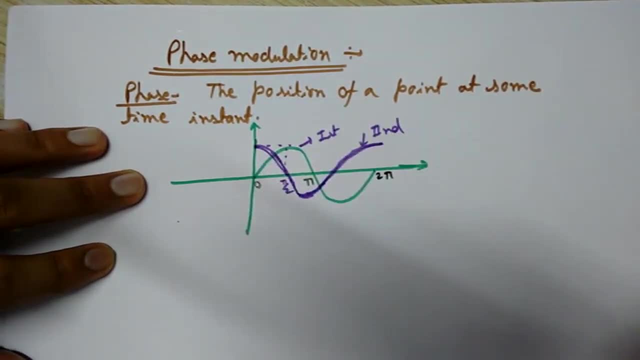 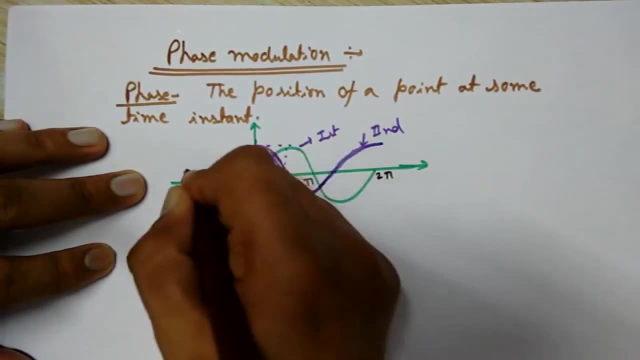 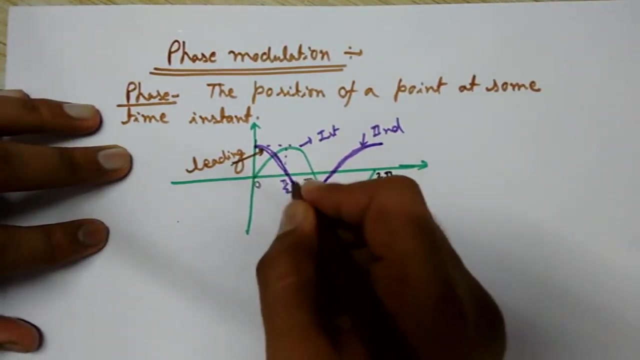 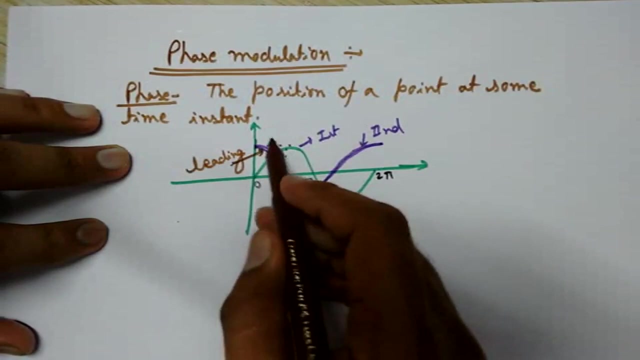 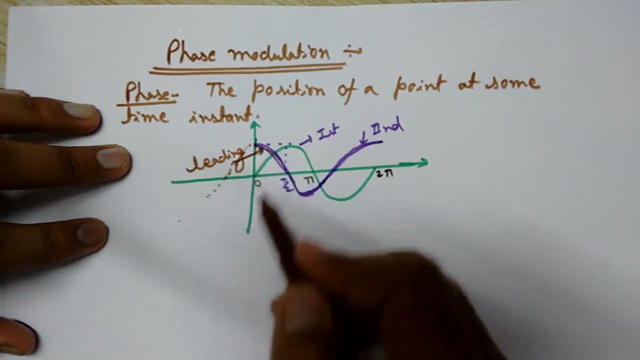 second, and you should know that this one is the leading waveform, this one Leading in phase by 90 degrees, or pi by 2.. As you can see, this wave has been moved horizontally, since, if you draw this, the form will be like this. I'm just making it with the help. 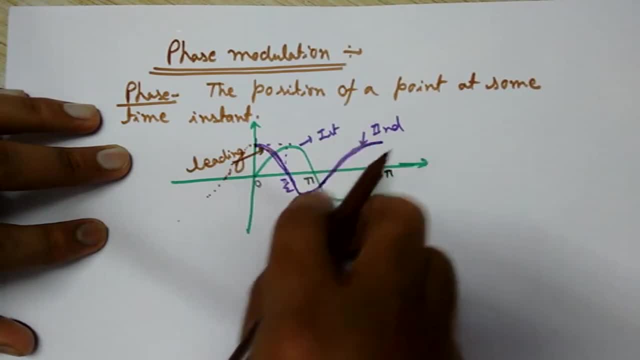 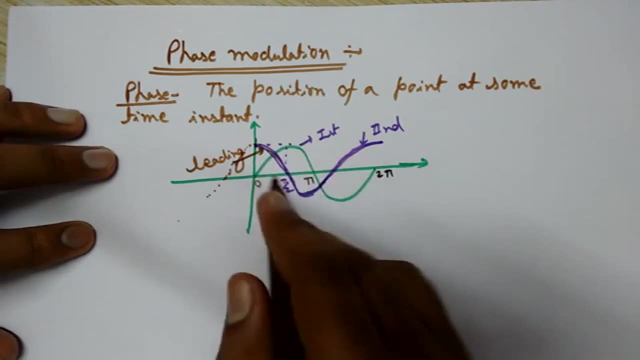 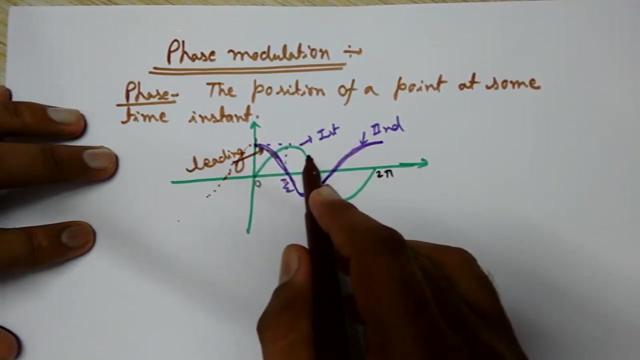 of dots. So this waveform, this shown in blue second waveform, is pi by 2 ahead of this first waveform shown in green. So this is the leading and this is the lagging. Sorry, green one is leading wave and the blue one is the leading wave. So this is. 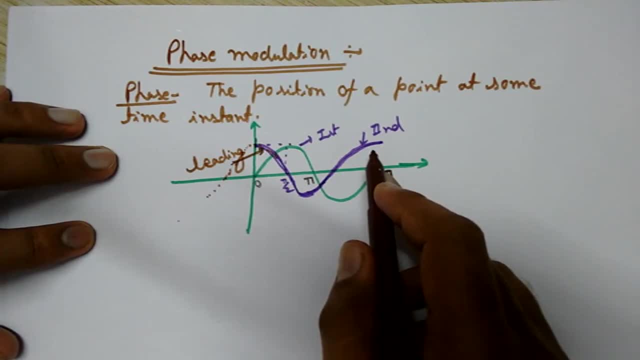 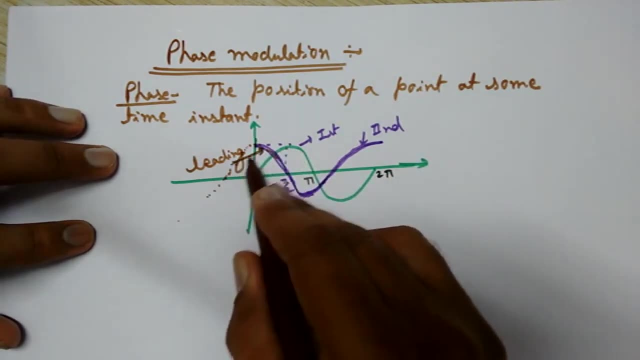 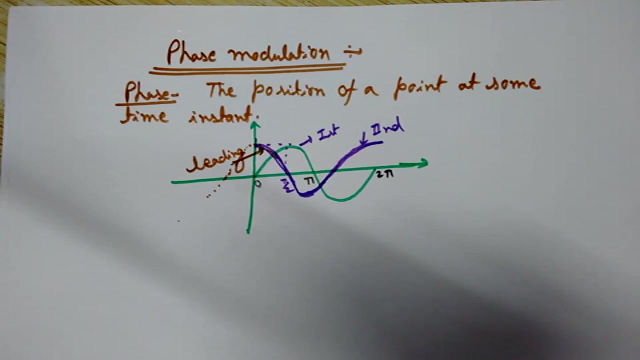 the leading wave and the green one is the lagging wave. Sorry, I just said it opposite. This blue one is the leading wave and the green one is the lagging wave. So these waves are called to be in phase quadrature because these are 90 degree phase difference. so these 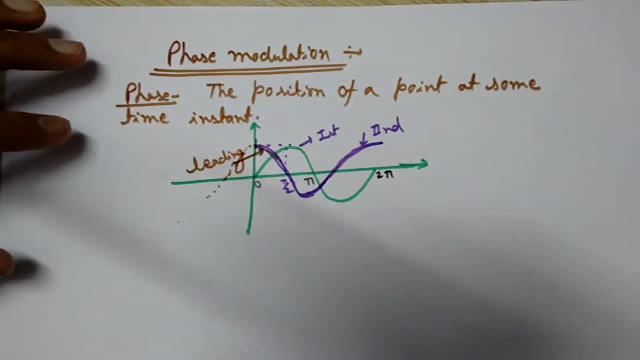 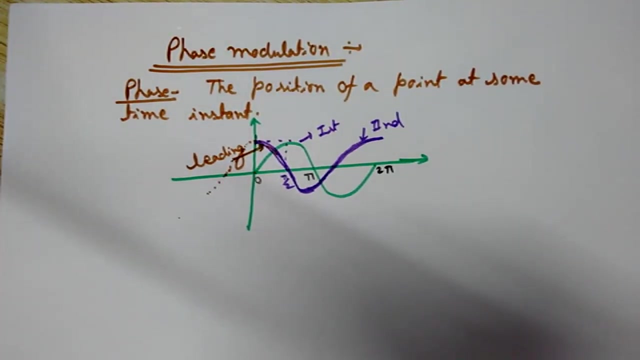 are in phase quadrature, But if they differ by phase difference of 180 degrees, like pi, then these are called in phase opposition. So now let's define the phase modulation. Let's come to our topic: phase modulation. What is phase modulation? In phase modulation, the instantaneous phase, 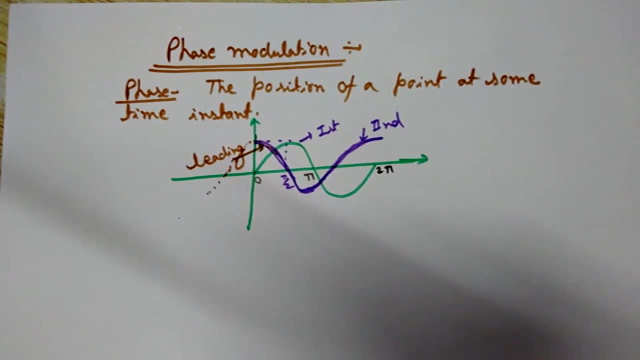 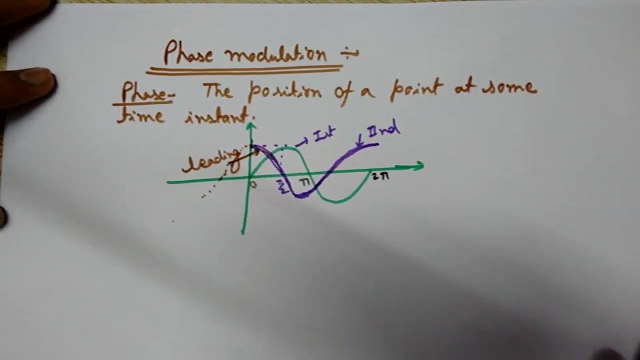 of the carrier wave is varied according to the amplitude of the message signal. okay, here we will vary the phase of the carrier wave, as we have seen in amplitude and frequency. we varied the amplitude and frequency of the carrier, so in phase we will just vary the phase of the carrier wave. so let's analyze the waveform of the phase modulation. 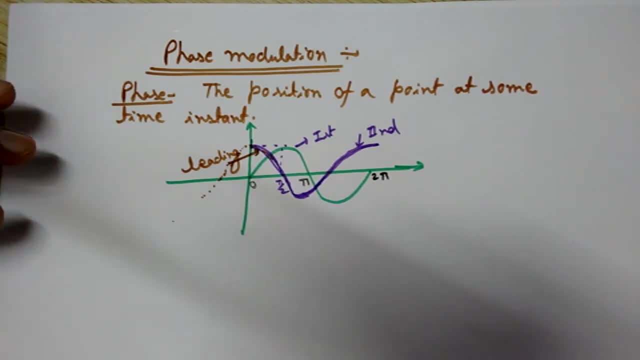 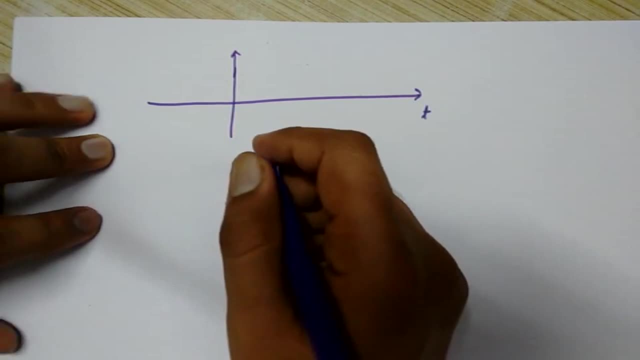 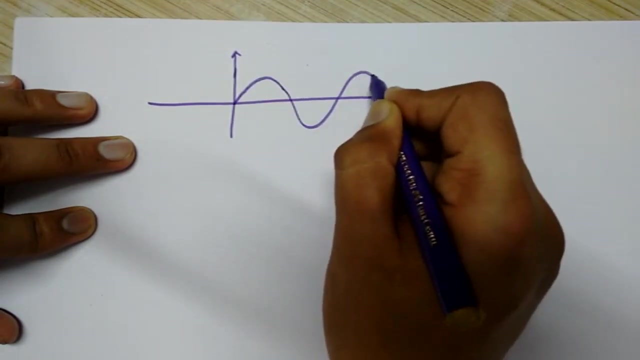 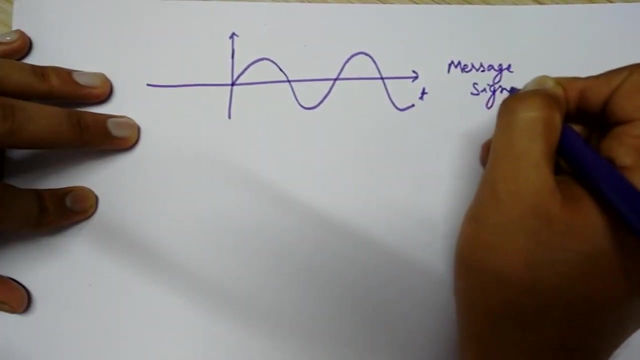 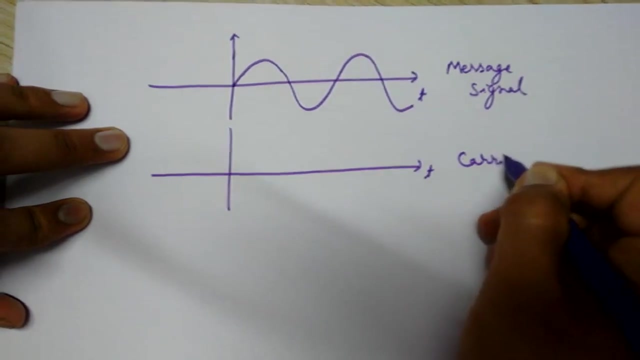 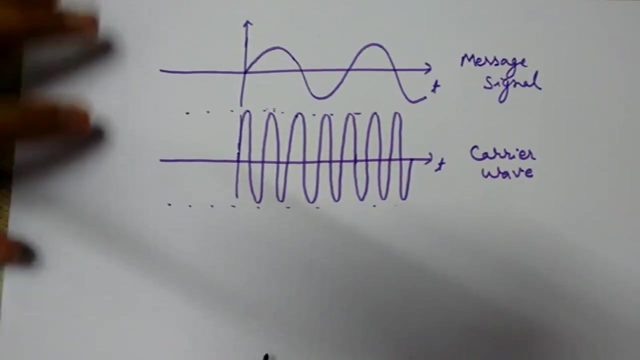 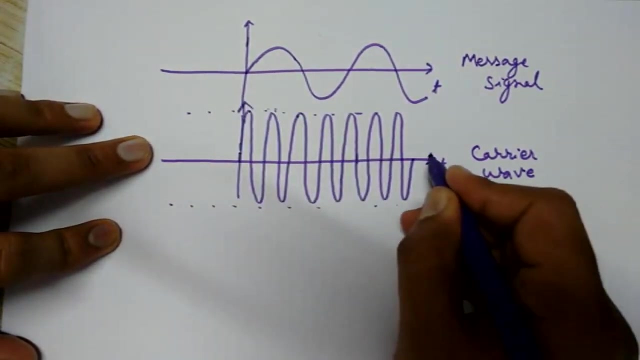 phase modulated here. if this is the, this is the time axis, I'm drawing the message signal. okay, this is the message message signal and this one I'm drawing here the the carrier wave. so now i'm drawing the phase modulated wave. only the phase of the carrier will be varied here, not the frequency. 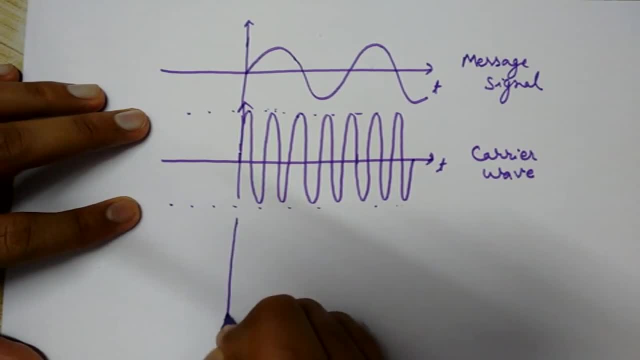 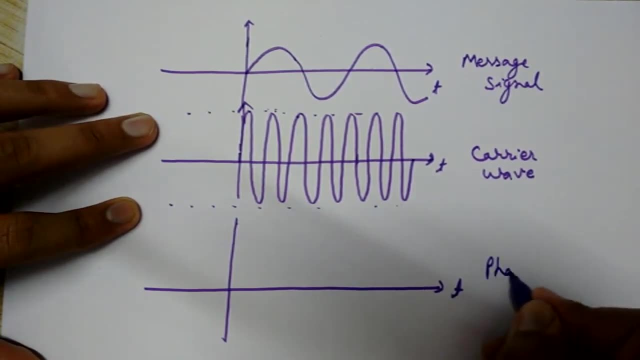 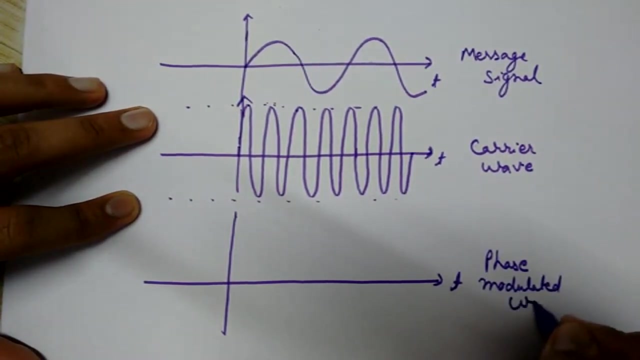 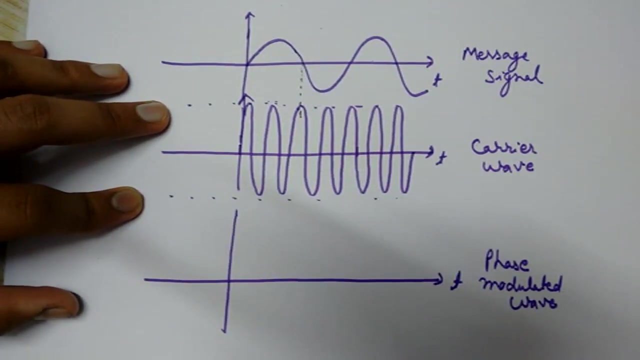 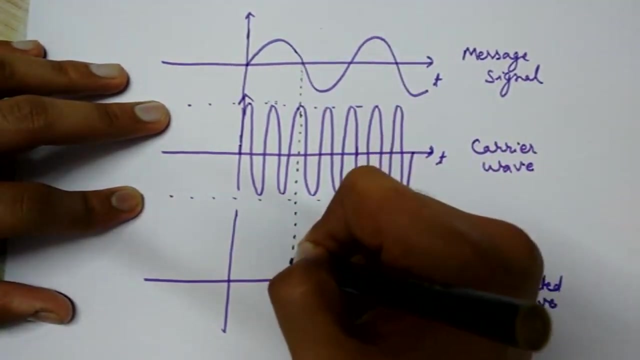 neither the amplitude, only the phase. the information will be contained in the phase changes. so the phase modulated wave i'm going to draw, so let's observe it. these are the. these are the times when the message signal cuts the time axis. i will show you its importance, why i'm drawing these lines. 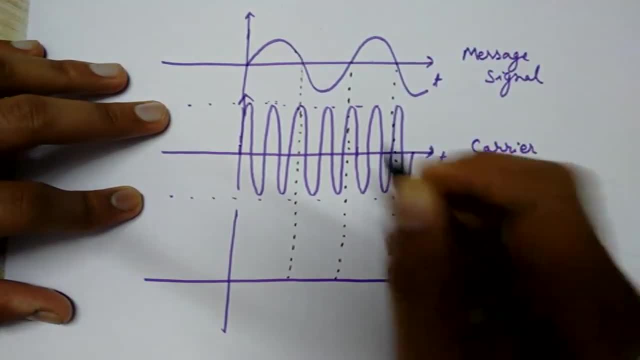 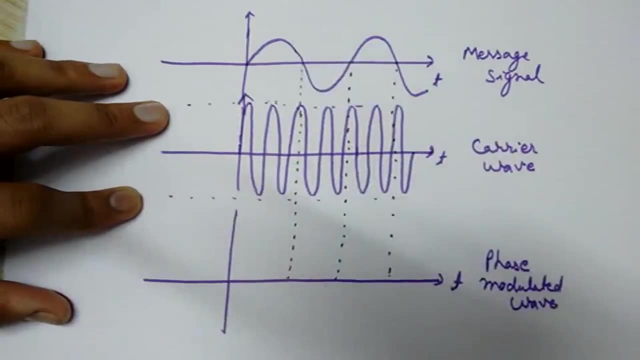 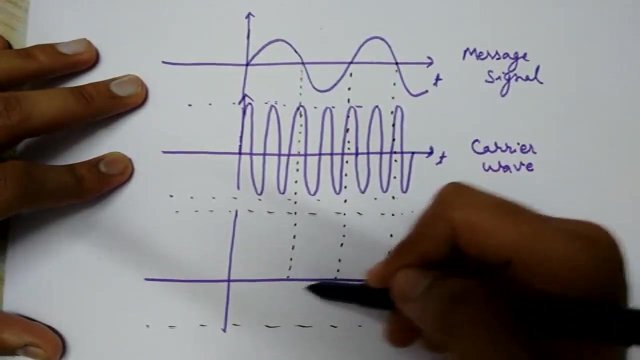 at this instance, the message signal cuts the axis. this, this, this point, this point and this point. okay, i've drawn vertical lines through this. how does this happen? at these instants, only at these instants, the phase will change. at these three instants in this diagram. 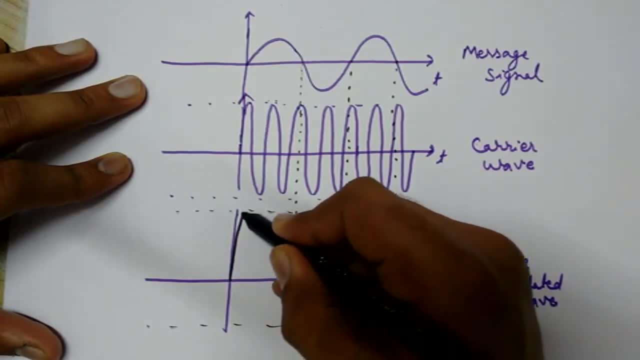 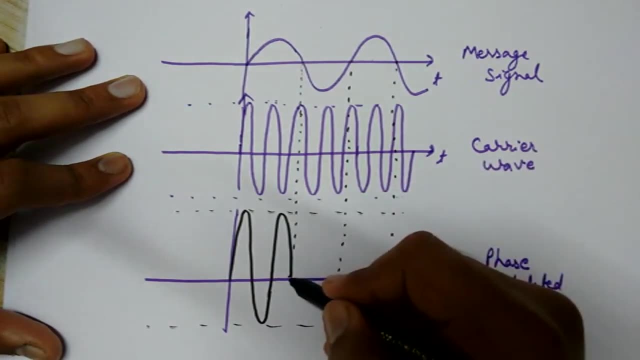 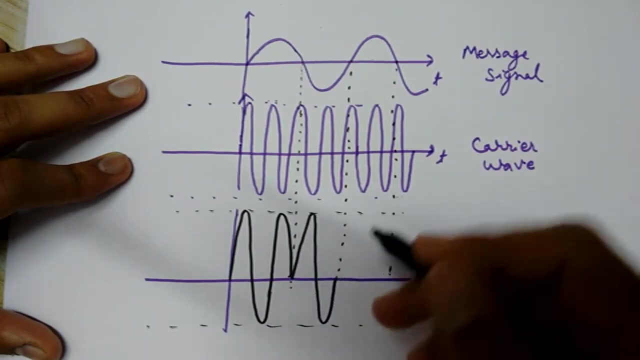 so how does this happen? okay, this, the original path was like this, but it goes in this direction again at this point. the original path was in this direction, but a phase change happens here and it goes. the same thing happens at this point. okay, i think it's clear. 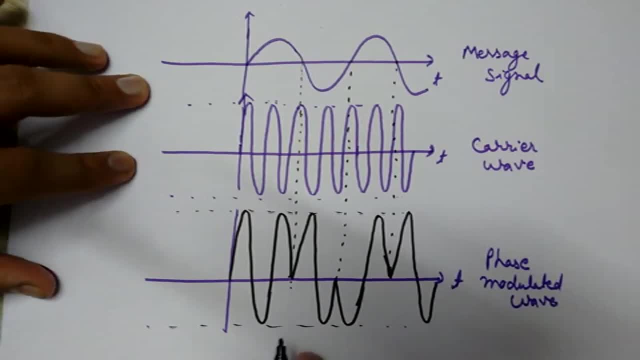 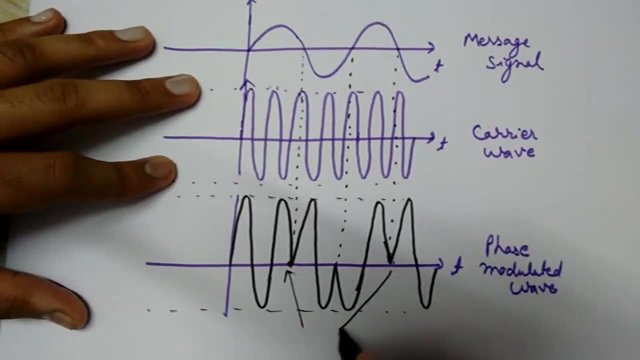 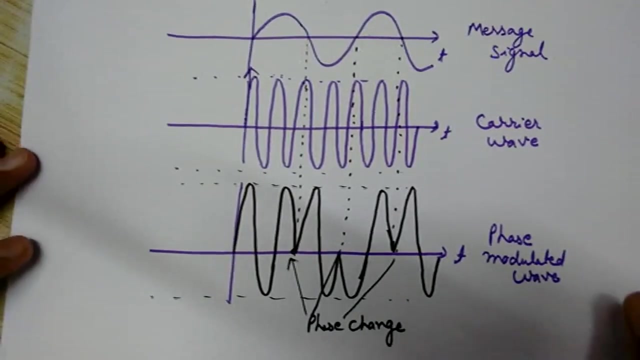 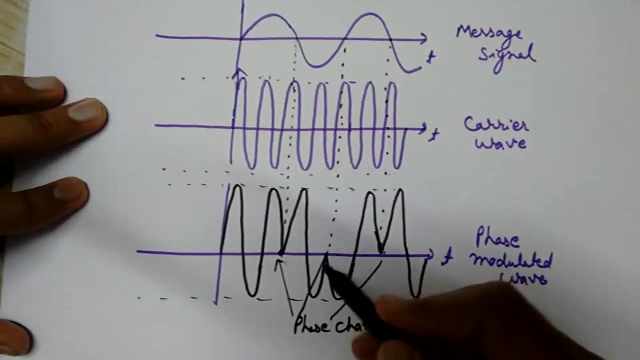 so these are the three points where the phase change happens. okay, the phase change has occurred. okay, these are three points. your phase change has occurred, okay. so for the phase, the change means just the horizontal shifting of this wave. we have shifted this wave, this, the original path was in this direction, it's. 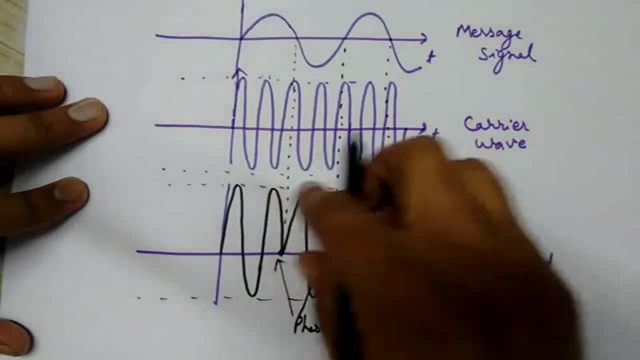 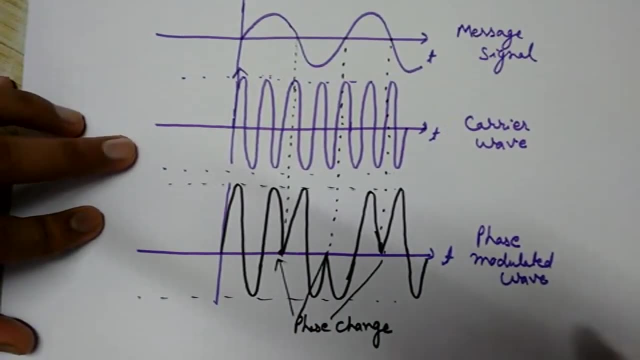 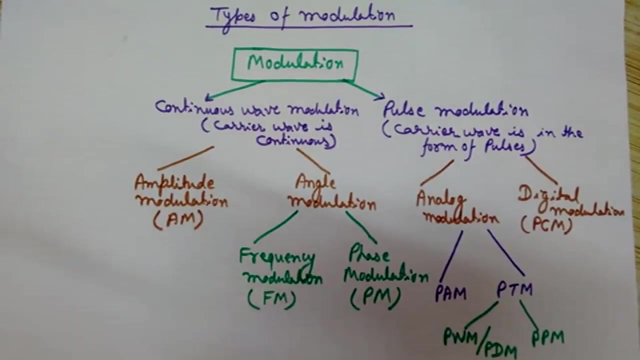 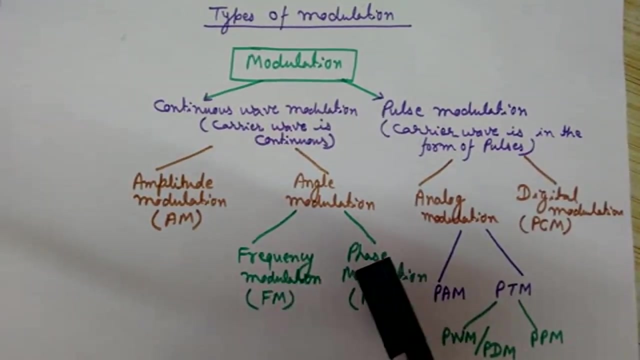 saved would have been like this, but we have shifted this wave in the horizontal direction, so this was the phase modulated waveform. so in this lecture we learned about various continuous wave modulation techniques, which includes amplitude modulation, am, frequency modulation and FM and phase modulation, PM. So this was all about continuous wave modulation, where the carrier wave 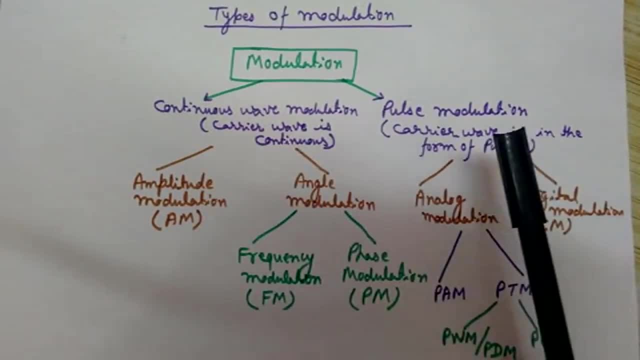 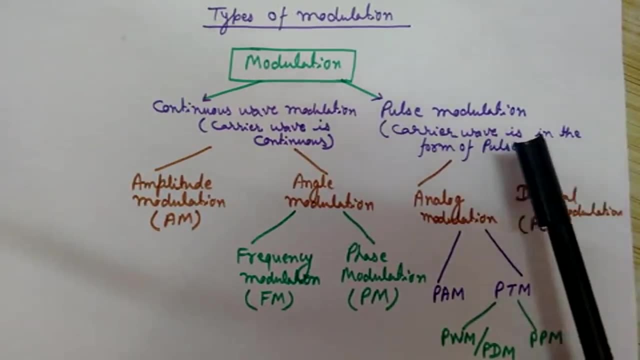 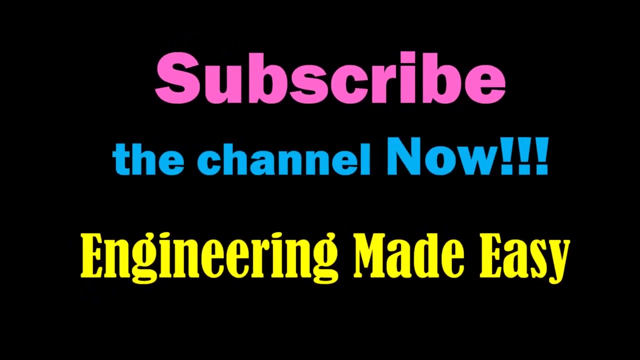 is continuous in nature. In the next video we will see pulse modulation, where the carrier wave is in the form of pulses. It includes PAM and PTM. In the next lecture we will discuss all these types this PWM and PPM Friends. for more such videos, you can subscribe my channel.